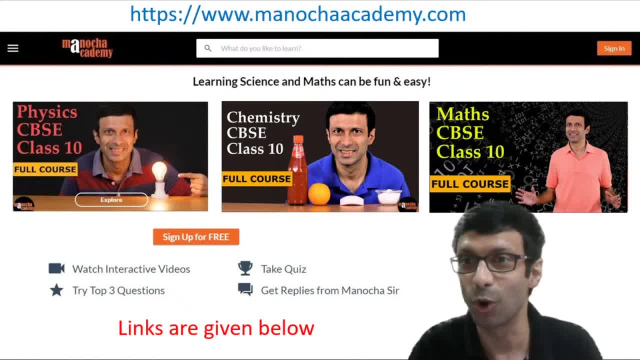 big discounts right now. So do check them out- They are full courses- and do share it also with your friends And guys. I'm excited to announce that because a lot of you gave feedback that you guys want Hindi classes also, So we've started more live classes on our Manocha Academy Hindi channel. 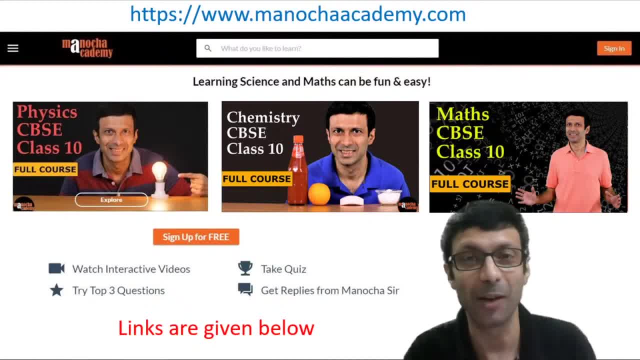 So just yesterday we had a class on our channel, Manocha Academy Hindi. So if you guys are interested, you can also subscribe to that channel in addition to this one. Okay, guys, and if you haven't hit the subscribe button for this channel, please hit it right now and click on the. 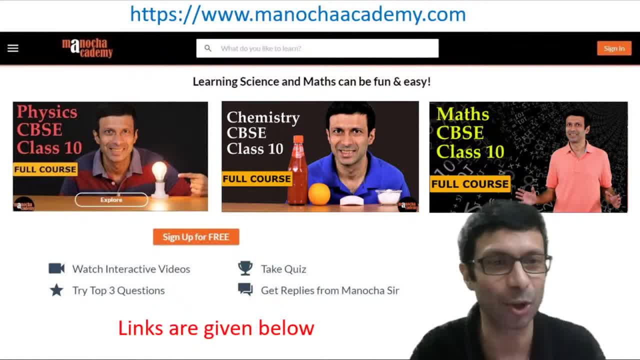 notification bell so that you don't miss any of our new videos. So if you haven't hit the subscribe button, you don't miss a single live class or the videos that we upload. All right guys welcome. welcome everyone, Great to see. good evening to all of you. Sorry if I can't take everyone's name here. 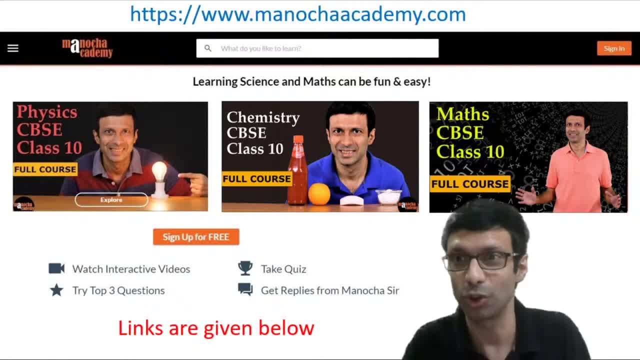 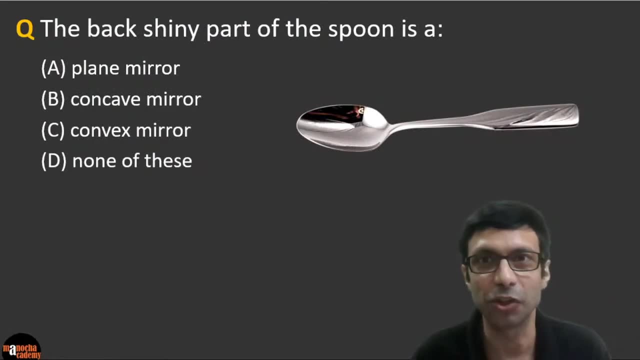 but make sure you do subscribe to our channel, So Manocha Academy. in this channel I'll be taking the English classes, and we also have Manocha Academy Hindi. All right, so let's go ahead and begin this quiz. I'm Sandeep Manocha and let's start this quiz, guys. So here's the first question. 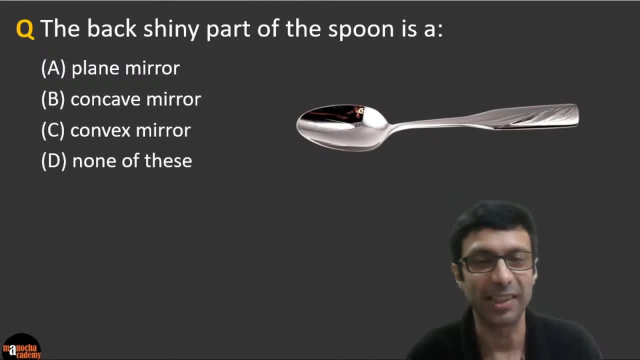 The back shiny part of the spoon. What is it? A plain mirror, a concave mirror, a convex mirror or none of these? What do you guys think Awesome? Come on, I want everybody to try here. So the back shiny part. 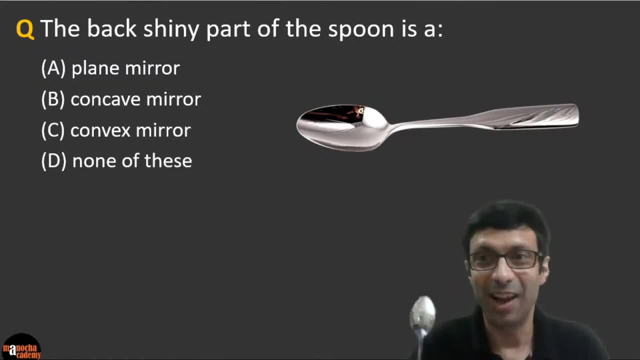 of a spoon. So, guys, next time you're eating your lunch or dinner, please, you know, pick up your spoon, right? So pick up the spoon and check. You know that the spoon has a curved surface and a shiny spoon is a reflecting surface, right. 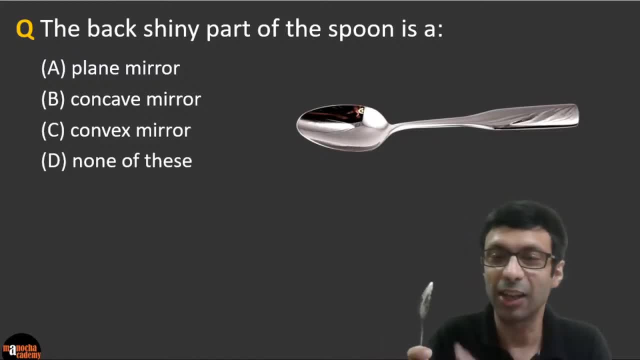 Guys. so if you take a look at a spoon, you know that it it has a curved surface on the front and the back side. and this question is asking the back shiny part of the spoon, Okay, so this is the front shiny part that I'm seeing here. and, guys, this is the back portion, Okay, so what type of mirror it? 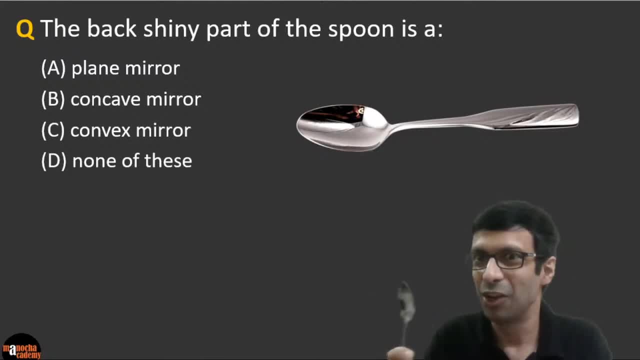 is. and the best way you can check, you know, by looking at yourself. So look at yourself in the back portion of the spoon. that is this one, right? This is the back portion of the spoon. So what will it be, guys, Come on. 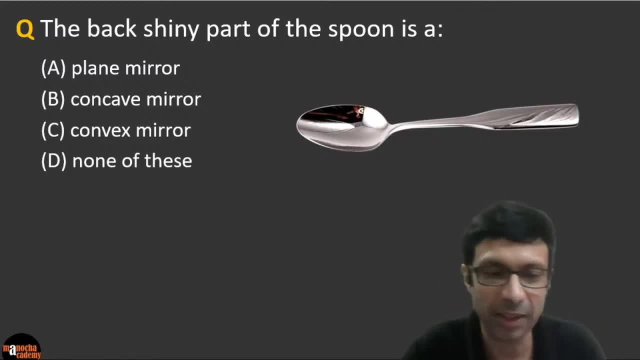 Is it a concave mirror, a convex or a plain mirror? So, guys, the answer cannot be plain, because we are talking about a curved mirror, right? You know, the spoon is carved in shape, so plain mirror cannot be the answer. So which one is it? So if you pick up the spoon and see yourself like I'm looking at, 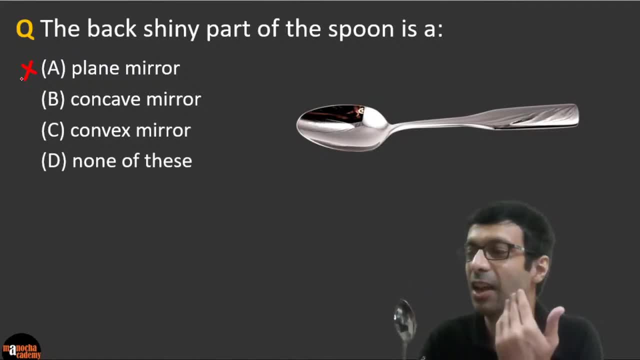 myself here, right? So guys, do this experiment after this class. Look at yourself in the spoon and no matter where you move it, you'll see that you're getting a upright and diminished image. But if you turn the spoon- Right front part- you can see an inverted version of yourself right. so in the front part there's an. 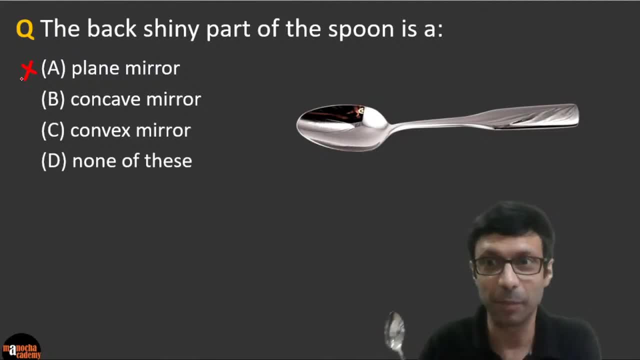 inverted version. that means it's a concave mirror. right there's an inverted image in the front part and in the back portion there's always a diminished and upright image right and it is a convex mirror and you can also feel it. you can see that it is curved outwards, it's bulging outwards, so excellent. 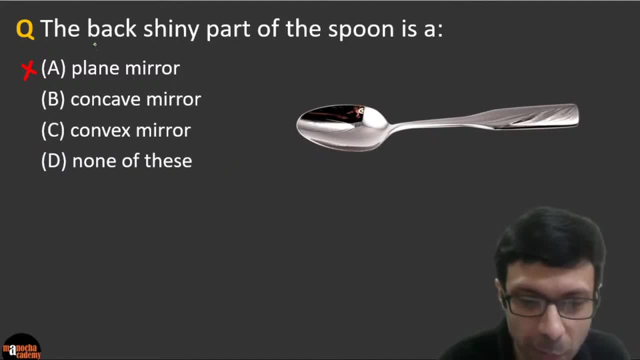 guys. correct answer here is: the back portion of the spoon is a convex mirror. so please remember that the front part, the front part, is a concave mirror because it curves inwards right, and the back portion, the back part of the spoon which bulges outwards, is a convex mirror. okay, excellent. 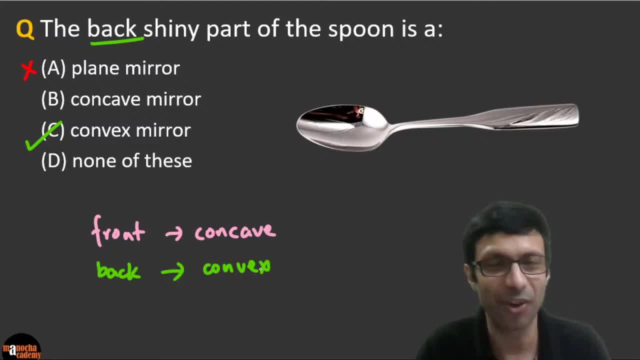 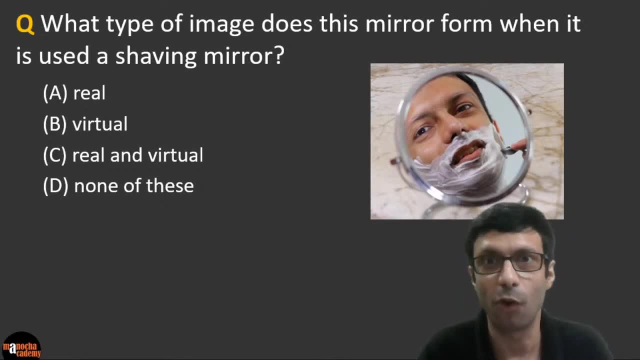 excellent. and, guys, if you haven't hit the like button, please hit the like button right now and let's move on to our next question: what type of image does this mirror form when it is used as a shaving mirror? so, as you guys saw in my thumbnail- you know i had this picture where i'm shaving, i'm using this mirror, right? 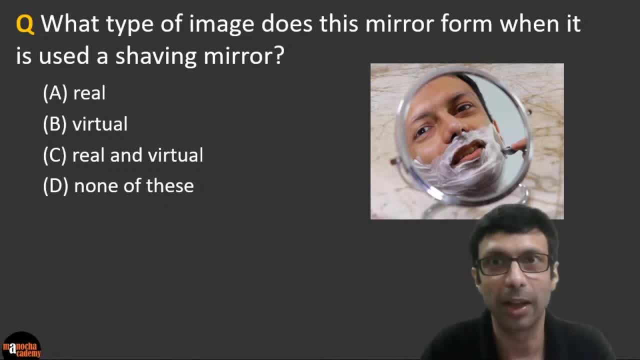 which is used called the shaving mirror. so what type of image is formed? is it a real image? is it a virtual image? a real and virtual image, or none of these? what do you guys think? so, come on, i want all of you to try excellent to see the response. 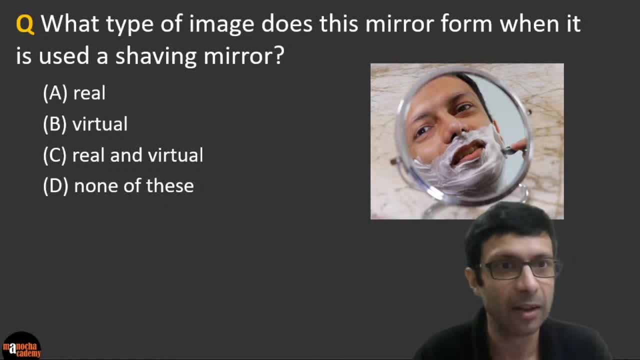 so a lot of you are saying b here, some of you think it's a. okay, some of you think it's c, real and virtual. so great guys, come on, please try, and doesn't matter if your answer is right or wrong. i want everybody to participate in this quiz, okay? so what is the answer here? so please take a look. 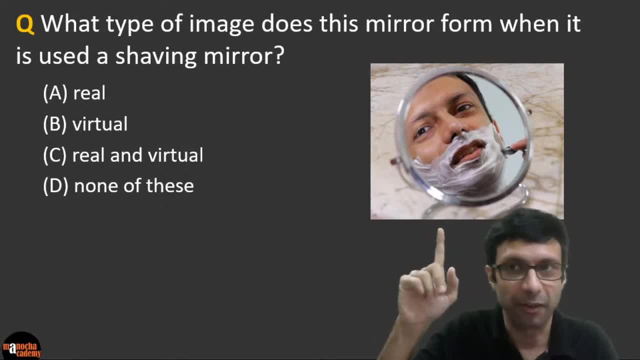 at this mirror, right? so i'm using a curved mirror here, right? because you can see that while i'm shaving? uh, is the magnified image of my face, right? my face is not that big, but when you see it in the mirror here it's a larger face, okay, so what type of image is formed in this case when you are using 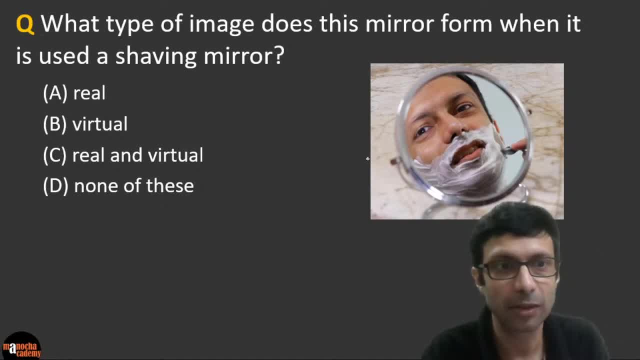 it as a right. so, first of all, what type of mirror is this? so what type of mirror is the shaving mirror? do you guys know what type of mirror is it? okay, great, great to see the answers. so this mirror, you know which is used as a shaving mirror. it is a concave mirror, right? 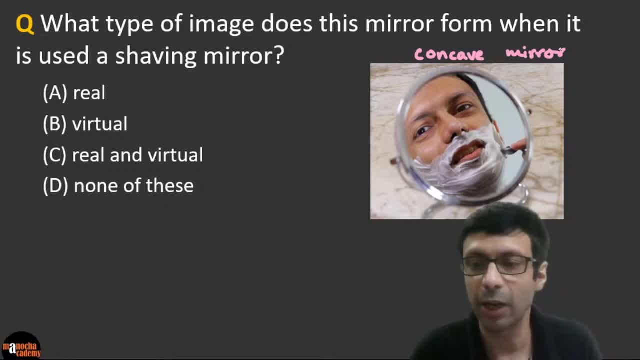 and when you're using it as a concave mirror. very good, lot of you are saying concave mirror, right? so when you use it as a concave mirror, you go close to it. and when you go close to it, it you know it gives a magnified image so it's easier to shave. or it's used as a makeup mirror, right. 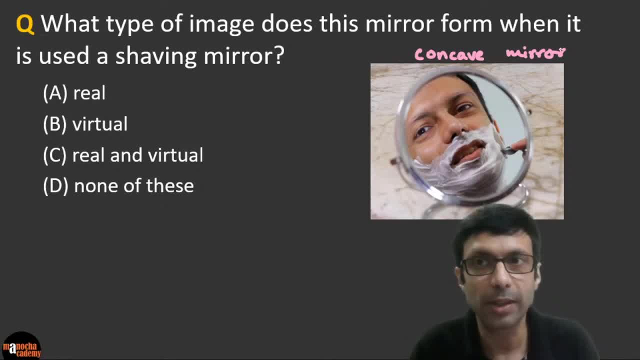 so it's easier to apply makeup. so now, what? what is the type of image formed here? come on, guys, and the answer is very easy. if you take a look at the my image here in this concave mirror is my image is inverted. okay, in this case, guys, don't. we are not talking about the general concave mirror. 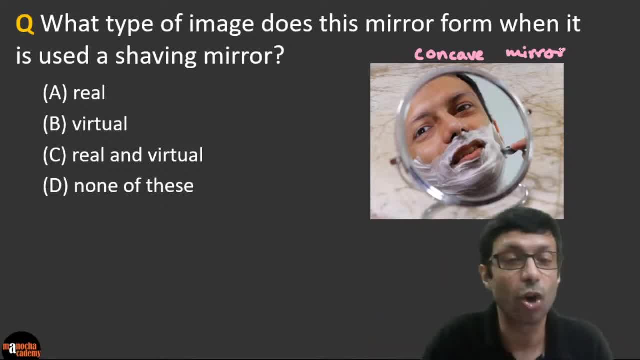 case, some of you guys are getting confused by that. in this case, in the concave mirror right in this, in this case of the shaving mirror, is my image upright or is it inverted? clearly, guys, you can see, my image is upright, right, my face is not upside down. it is upright here. it is not inverted. 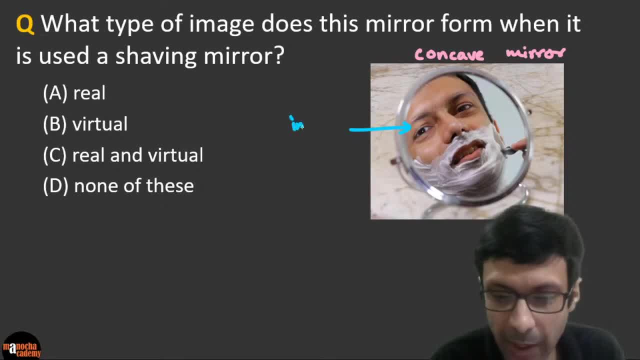 so all of you can see that the image here, right, my image is upright because it is not inverted, right? and which type of images are upright, virtual or real? come on, guys, can you tell me excellent, excellent, right? i see now a lot of you are saying virtual, right, because you know that is the rule: virtual images are upright, right? 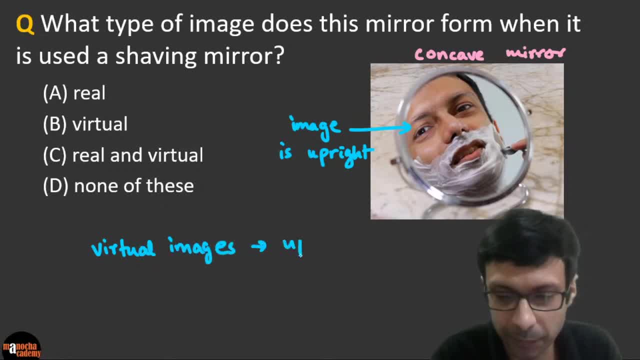 so virtual images are always upright, but really images, right. real images, they are inverted, because the rule is virtual and upright real images, they are always inverted. okay, so the correct answer here is: since it's an upright image, in this case a concave mirror can form both. you guys know it right, it can form real and virtual, but in 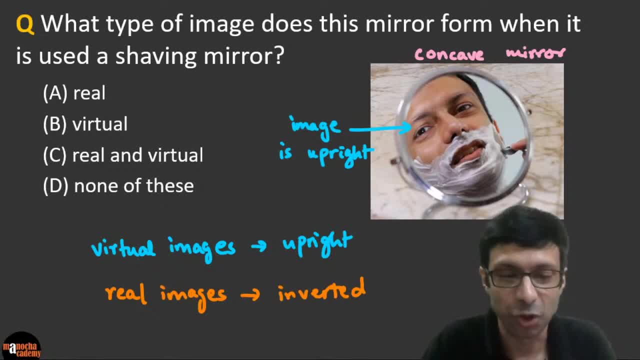 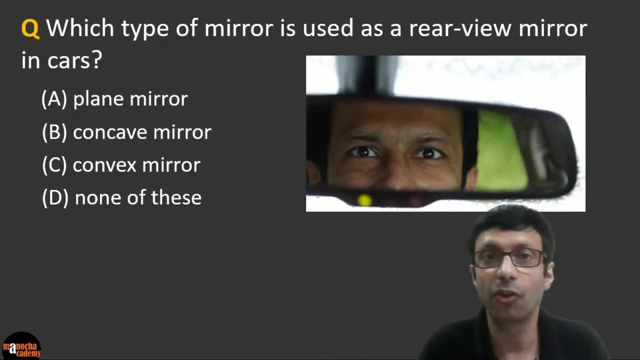 the shaving, shaving mirror case. it's forming an upright image, so the answer is going to be virtual. right, that's the correct answer, because it is virtual and upright. excellent, guys, excellent, fantastic. let's look at the next question. which type of mirror is used as a rear view mirror in cars? so, guys, you know, in the cars, right on the 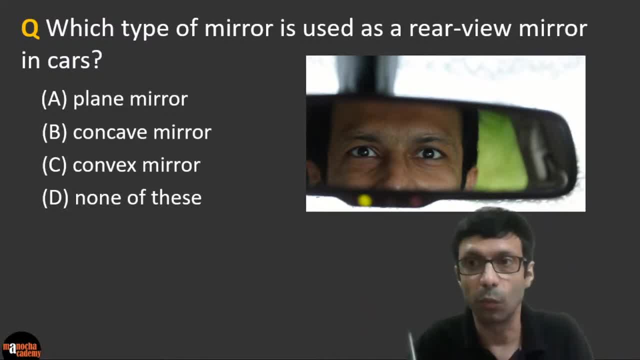 vehicles. they have this rear view mirror so that you can easily, while driving, you can see what is behind the car right, the cars or the road behind the car or the vehicle. so what type of mirror is used as a rear view mirror? come on, is it a plane, concave, convex, or is it none of these? 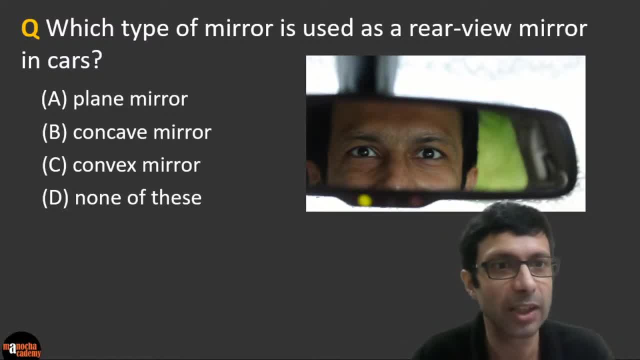 what do you guys think? so animesh says convex mirror, bindu here says convex. what do you guys think? mandip mandal also thinks convex. right, even satya singh says that: come on, i want everybody to try. okay, excellent, guys, excellent. so it is actually not a plane mirror, because a lot of people you 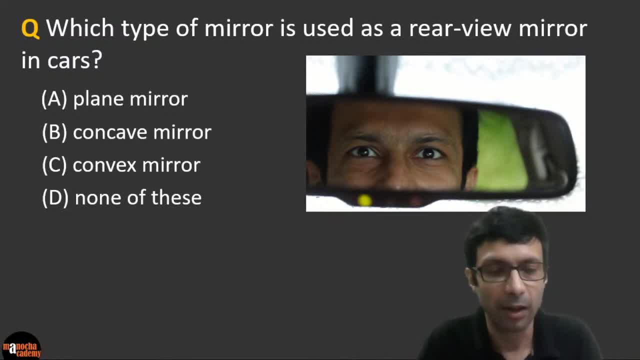 know when they look at this they think, oh, you're looking at a plane mirror. the answer is not plane, because this mirror is slightly curved, very slightly right. you can next time you know when you're in a vehicle you can see right. in a bus it's a little more evident because the buses they have big rear view mirrors. in a car, the rear 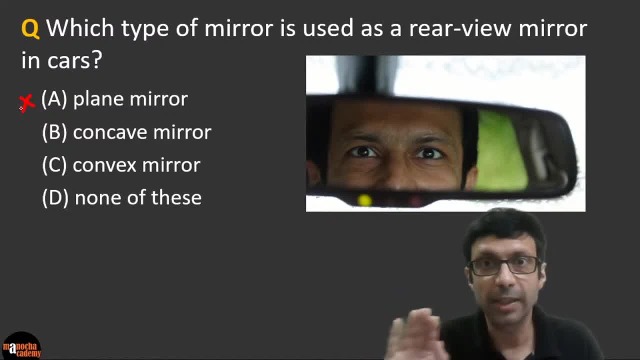 view mirror is smaller right, so you can see that the mirror is slightly curved. these types of mirrors are slightly curved. they are slightly curved, so they are clearly curved mirrors right, not a plane mirror. so which one is it? concave or convex? excellent, the answer is convex. so why do we use a convex mirror? so who can tell me why is a convex? 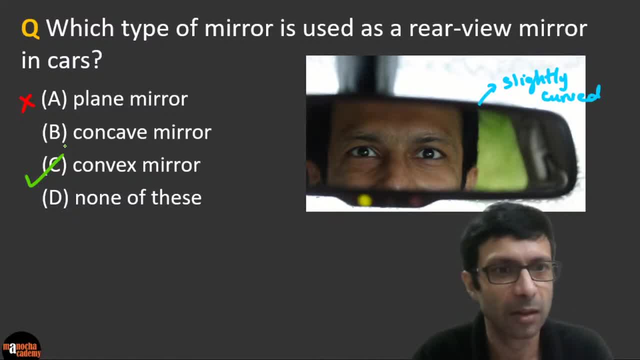 mirror used. why not just use a plane mirror, guys? so why do you use a convex mirror in a car, in the rear view mirror of a car? why is a convex mirror used? why not use a plane mirror? who can tell me- come on, excellent, i see pushkar gave the right answer. larger field of view even. 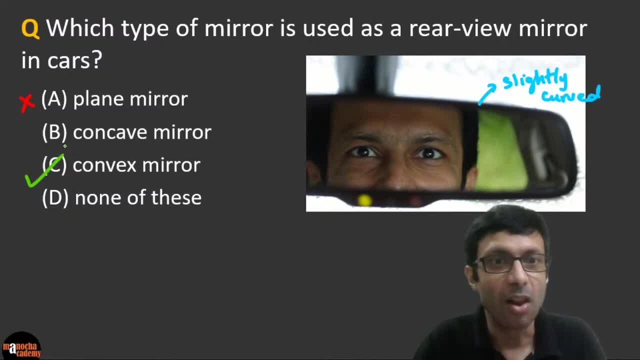 gotham says that: superb, guys, so that you get a larger field of view, not magnification. you don't want magnification, guys. very important concept: a convex mirror, right? so if you took, take a look at a convex mirror, it gives you a greater field of view, right? so for the driver, he gets a wider. 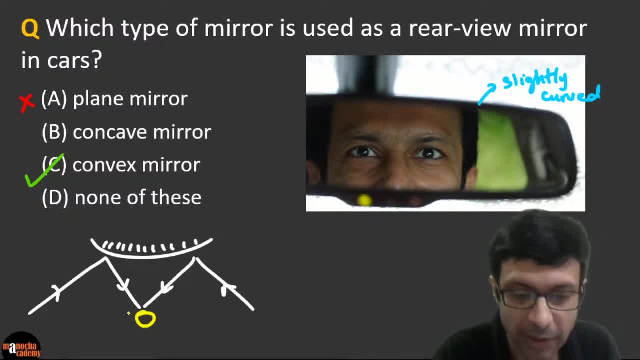 viewing angle right. so if this is the driver here you can see a convex mirror will give what we call as a greater field of view. greater field of view, okay, very important, excellent guys. excellent because it is a diverging mirror. excellent. a convex mirror, you know, is a diverging mirror. 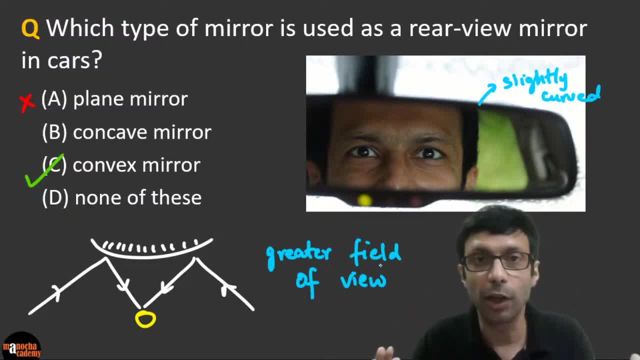 it gives a greater field of view. so, or a larger field of view so that you can see more of the road behind you. you can see the cars from a more, a larger angle. all right, excellent, excellent, guys. so that's the correct answer. let's go to. 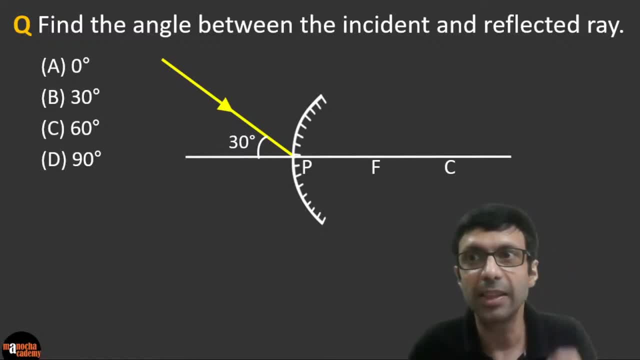 the next question: find the angle between the incident and reflected ray in this diagram. so come on, guys, you need to find the angle between the incident ray and reflected ray, and i hope all of you have your pen and paper ready, right? so please draw this diagram and try. 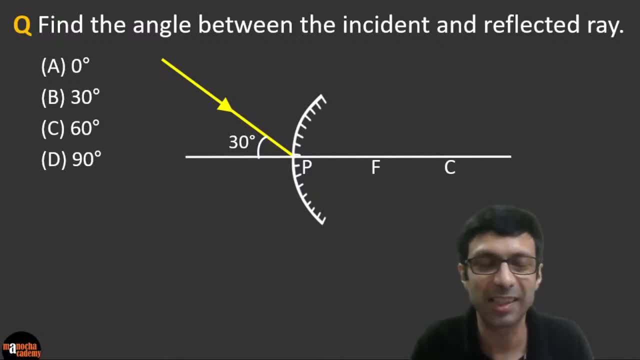 to work out the answer. please don't do the. you know questions in physics, chemistry and maths, you know just mentally. please draw the diagram and tell me what will be the answer here. okay, some of you are saying 30, some of you are saying 60. come on, guys. 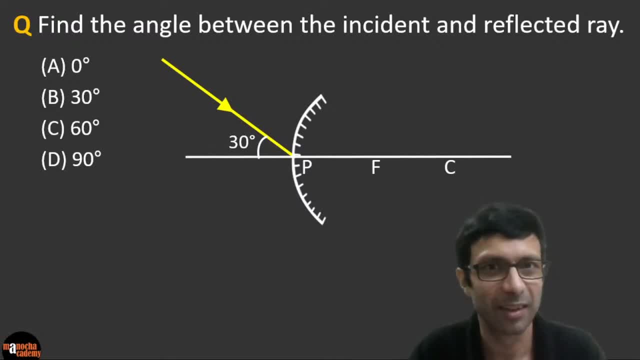 decide, and i want all of you to participate. so what type of mirror is this, guys? clearly you can see that this is a convex mirror, right? because this is the, this is the non-reflecting surface, so the mirror is bulging towards. so this is clearly a convex mirror, right? and what happens to this reflected ray? so they are asking the angle. 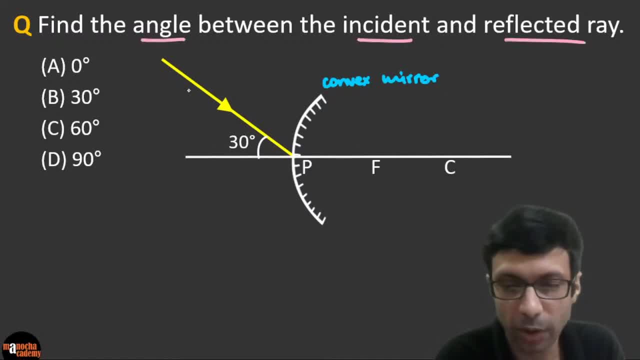 between the incident and reflected ray. so this is the angle between the incident and reflected ray. so So this is the incident, ray guys, It is incident on the mirror. And how do we draw the reflected ray? So you need to use the laws of reflection, the rules of reflection for concave and convex mirrors. 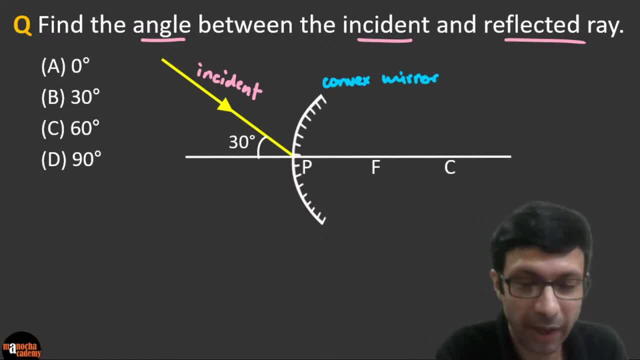 So what rule will you apply? Can you see? it is hitting the mirror at the pole. The center of the mirror is called the pole, And so this obeys a very simple rule: that it will reflect off like this. Okay, so it will get reflected like this: Oops, the ray vanished magically, right? 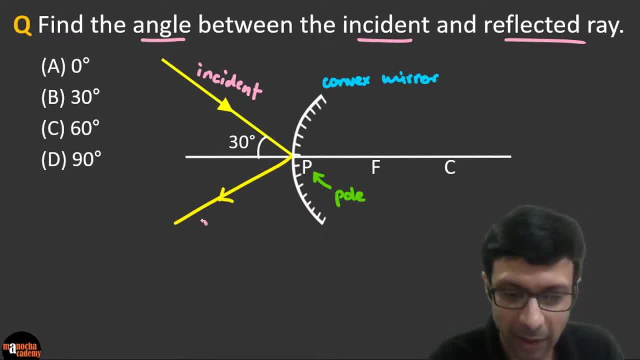 So this is the reflected ray here, guys, And what is the rule say? The rule says that the angle of reflection at the pole right The angle of incidence. you guys know that this is the angle of incidence- 30 degree- and the angle of reflection will also be the same. 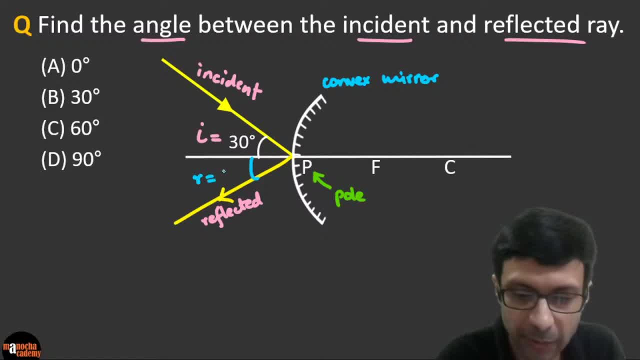 So angle of reflection here is going to be 30 degrees. Okay, because this is the rule. Please, you can read it in your books, right that at the pole, whether it's a concave or convex mirror the incident ray. when they hits the pole, the angle of incidence equals angle of reflection. 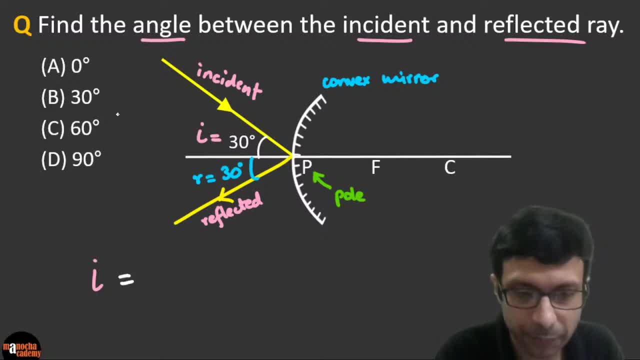 Very important angle. I equals angle R. I equals R at the pole right. So what is the angle between the incident and reflected ray? Now, it should be easy. right, The angle between the two rays. can you see? it is going to be 30 plus 30.. 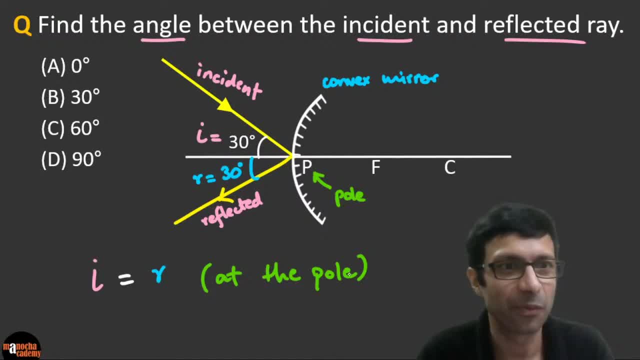 Excellent, right, 30 plus 30.. Fantastic, I see. Arjun has the right answer. Excellent, guys, Very good. Arush has the right answer. So it's just going to be 30 plus 30.. The answer is 60 degrees, because this angle we are talking about right. 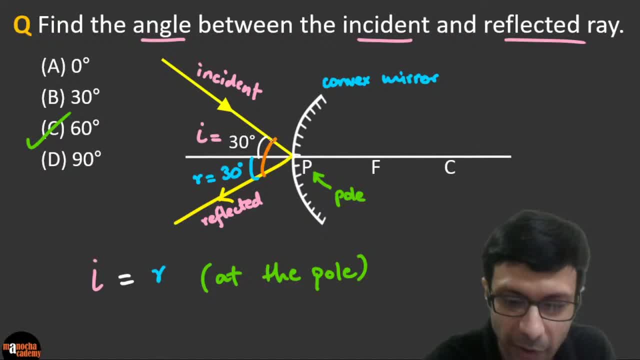 The angle between the incident and reflected ray. So the angle is going to be basically equal to the one we are interested in. It's going to be I plus R, I plus R, which is 30 plus 30. So our final answer is 60 degrees. 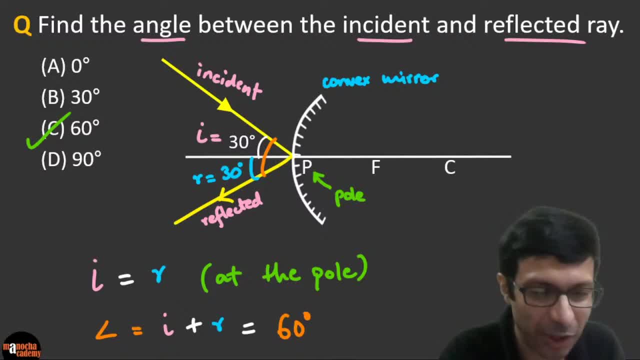 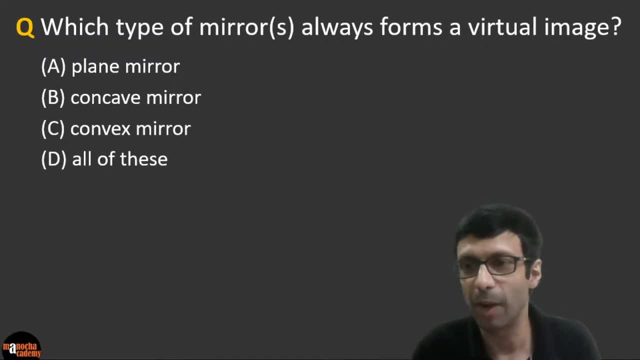 Fantastic, Awesome. Let's go to our next question, guys. Which type of mirror or mirrors always forms a virtual image? So here you can have multiple answers. So come on, all of you try. And, guys, if you like our live classes, please do check out our website, Manochacademycom. 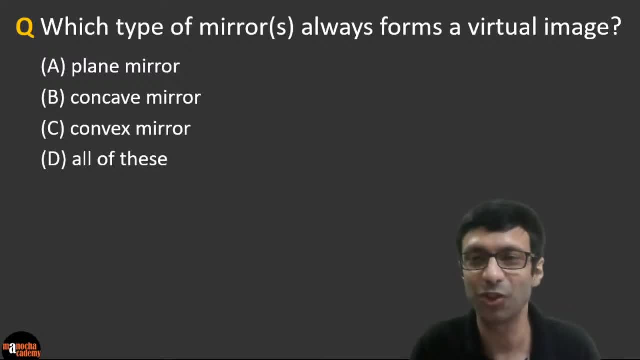 I take more live classes there on physics, chemistry and maths, So do check it out. And if you haven't subscribed to our YouTube channel, Manochacademy, please subscribe right now. Okay, And click on the notification bell so that you don't miss any of our videos or classes. 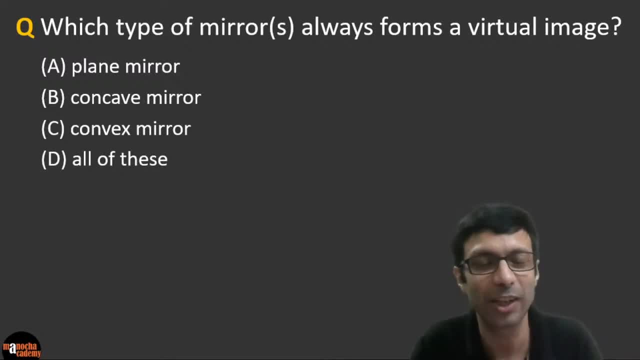 Okay, And guys also hit the like button. Great to see more than 250 likes for this class. I want all of you to hit the like button if you're enjoying the class. All right, Thank you guys. Thank you, Thanks a lot. 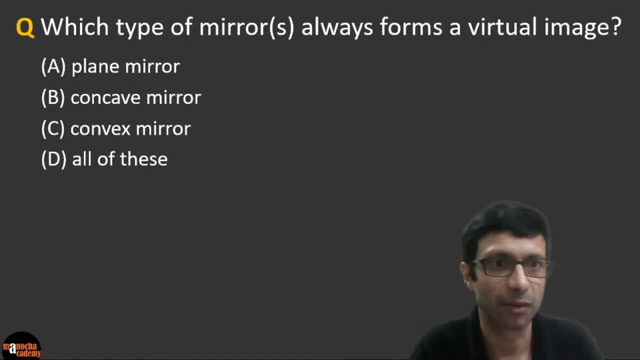 Come on, What is the answer here? Which type of mirror or mirrors? Right, What do you think? Always forms a virtual image. Okay, So very good. So when you comb your hair in front of a plain mirror, you see that always it forms a virtual image. 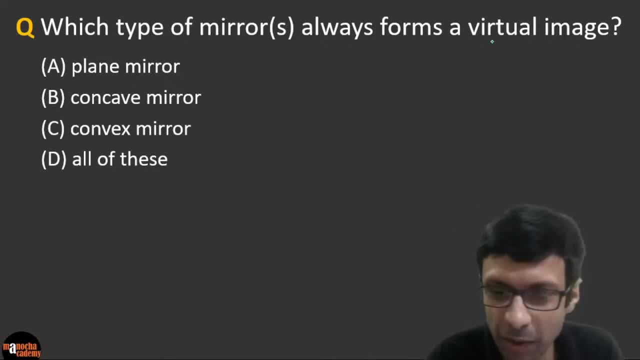 Have you ever seen yourself upright? Because, guys remember, virtual images are always upright, Right, So it's always virtual and upright. So you know that a plain mirror forms a virtual and upright image, Right? Okay, Concave mirror. This is a special mirror. 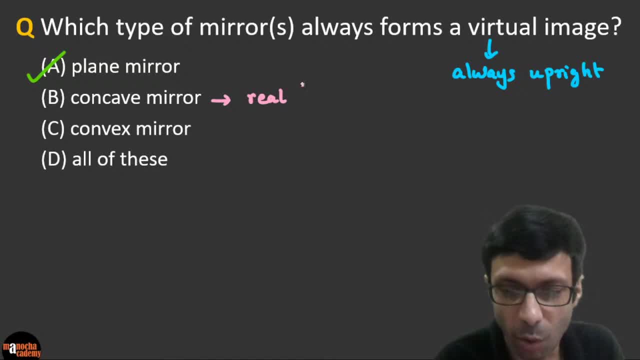 It can form both. It can form real or virtual images. Okay, So this is not going to be the answer. Right Convex mirror, Right, The mirror that we talked about. you know, in our rear view mirror, this guy always forms. 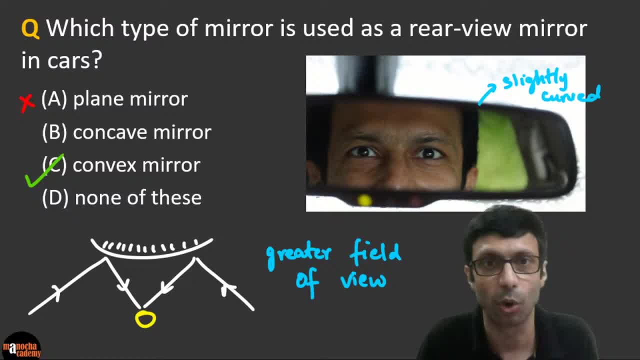 virtual and upright, because the driver doesn't want to see inverted image of the road, Right, I mean, there'll be an accident, It will become dangerous. So always in a convex mirror, whether it's in the rear view mirror or the side view mirrors. 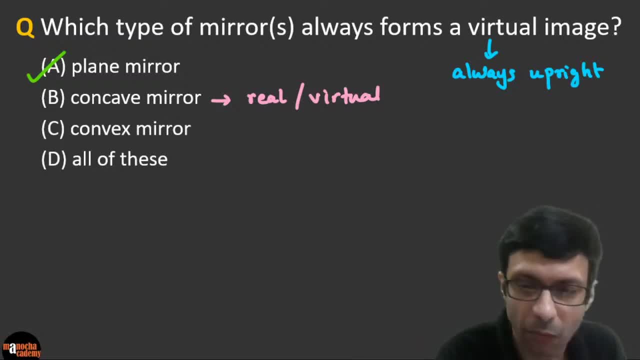 convex mirror. they always give a virtual image because it's virtual and upright. Do you guys agree? So excellent, Excellent, Right. So the answer it won't be all of these guys. The answer is going to be A and C here. 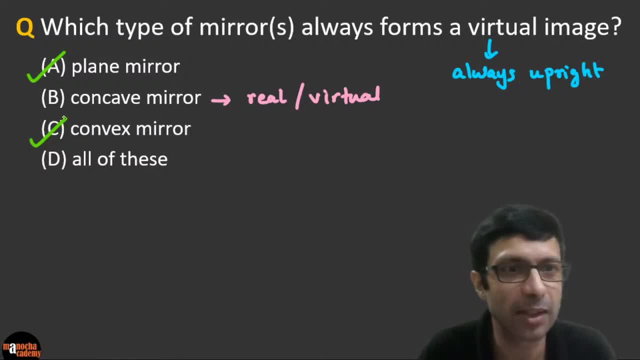 Okay, Very good, I see Neville also has the right answer here. A and C Right. Okay, Very good guys. A and C Right. Swati also has the correct answer. So it is plain mirror and convex mirror that can form virtual and upright image. 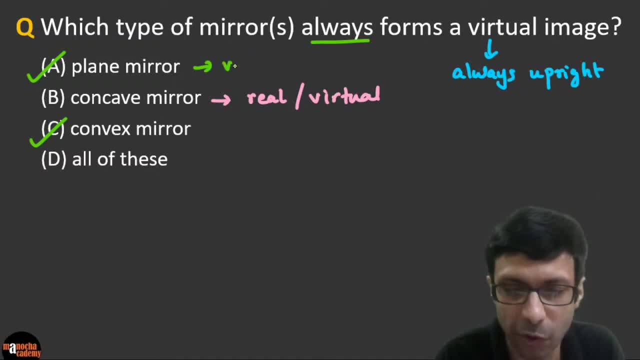 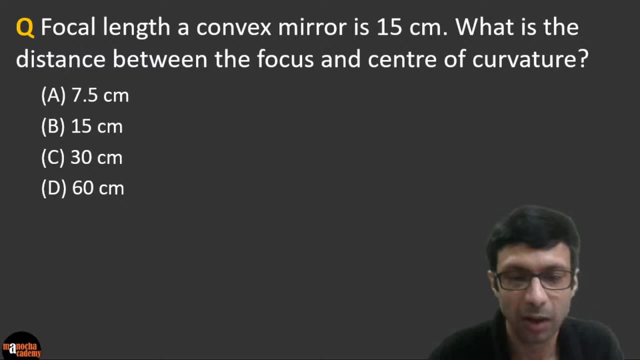 Okay. So if you look at these mirrors and they always, always give a virtual image, and this one, too, Always Okay. So convex mirror is the simple one in the syllabus. It always gives a virtual and upright image. Excellent, Let's go to our next question. 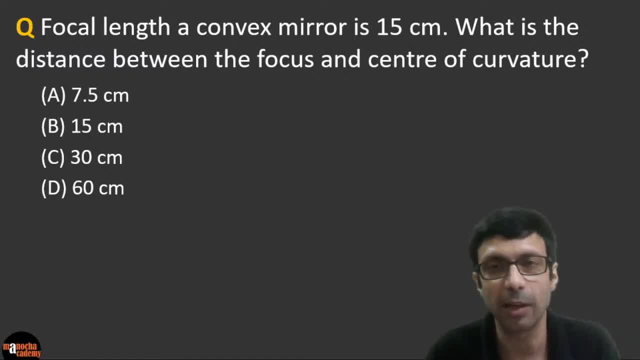 Focal length of a convex mirror is given to us as 15 centimeters. Now the question says: what is the distance between the focus and the center of curvature? And, guys, if you get questions like this, what is the focus? What is the first thing you should do? 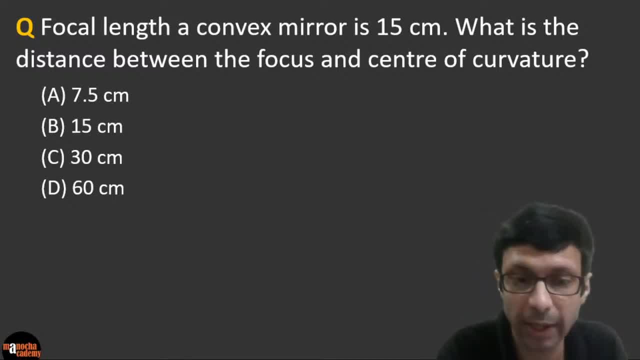 Please draw a diagram. Please visualize physics with a diagram. Okay, So I'm going to draw a diagram here, since it says convex mirror. Okay, I'm not a great artist, So you know, just excuse me if my diagram isn't that great, but let's sketch it out. 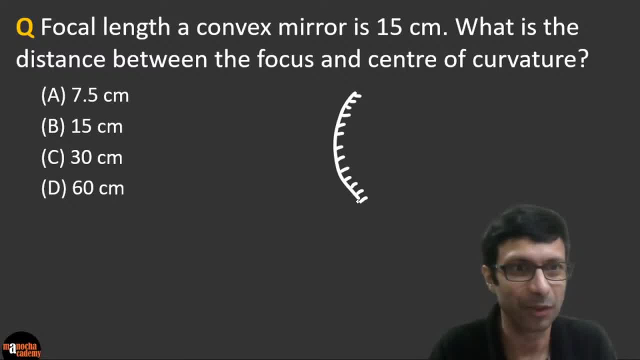 here. So this is a convex mirror and this is the back portion. right, That's the backside of the mirror, Okay, And always remember to draw the principal axis here. So, guys, you know that this point is going to be the focus. 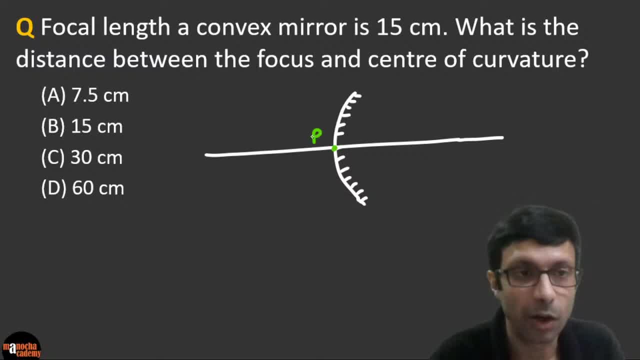 Okay, This is the pole right, The center of the mirror. Now, where will the focus lie? on the left side or the right side for a convex mirror guys? So you know, we have drawn a convex mirror here, Okay. 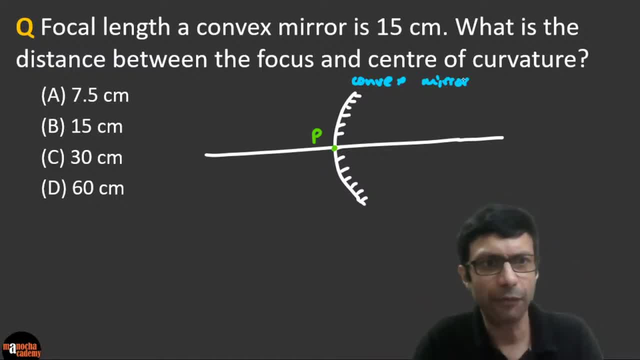 Where will the focus lie for this mirror? on the left or on the right? What do you guys think? Come on, All of you tried Very good, Great to see the response. Everyone's trying the answers here. Excellent, Excellent, Right. 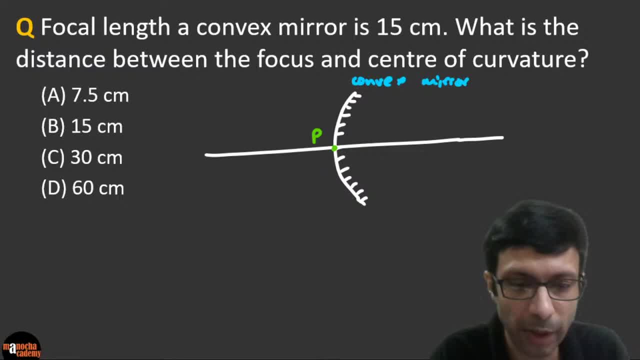 So here, very good, It will lie on the right, because you know that this mirror, it curves like this right. So that's why it's called a spherical mirror, because it's part of this big sphere. So what is the center of the sphere called? or the mirror? 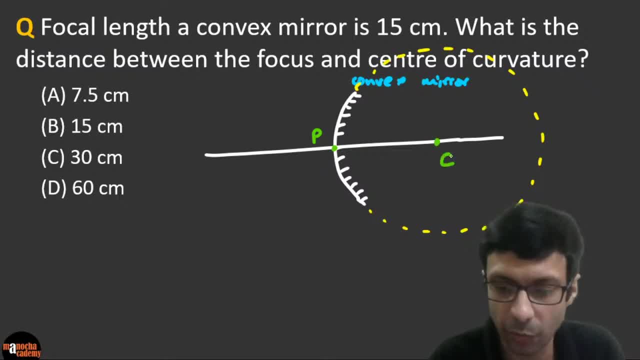 It's called, you know, the center of curvature. So, guys, do you agree? the center of curvature is going to lie here? I'll write pole over here: P right, The center of the mirror, center of curvature, will be here, right. 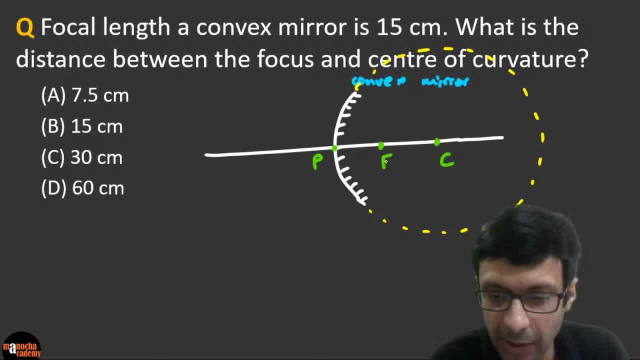 And the focus will be exactly between the P and C. P and C, the pole and the center of curvature. Clear, All right. So now, what have we been given? Focal length right, Focal length F is given as 15 centimeters. 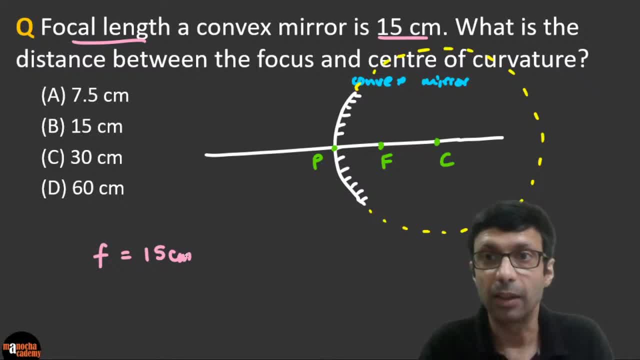 So F is given to us as 15 centimeters. Focal length means the distance from pole to focus. Okay, So distance from pole to focus is given to us as 15 centimeters. Do you guys agree, Right? And what do we need to find here? 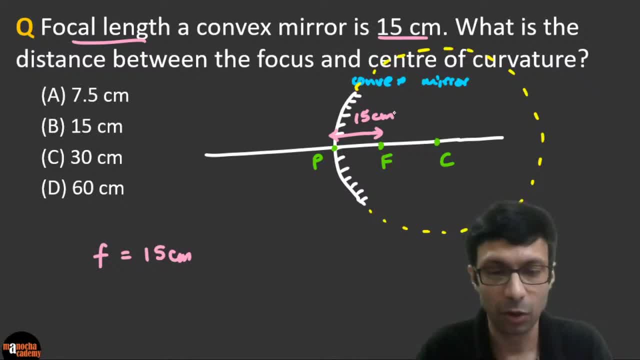 The distance between the focus and center of curvature. So, guys, please clearly mark it in your diagram. We need to find this distance between F and C. So see, now the visualization is so easy. If you have drawn a diagram, guys, please draw a diagram in physics. 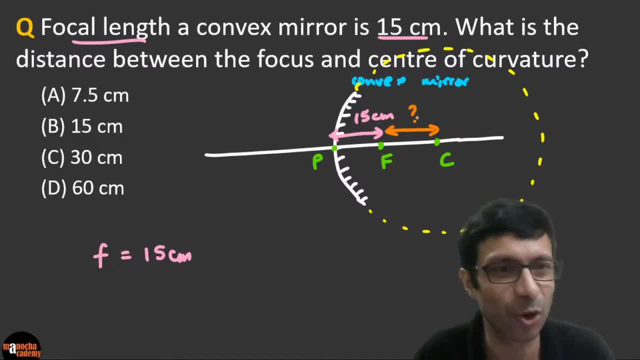 It's all about visualization. Okay, So what do you think is the answer going to be here? Awesome, Awesome to see the response. Okay, So Tanishq is saying 15.. What do you guys think? Shivam is also saying 15.. 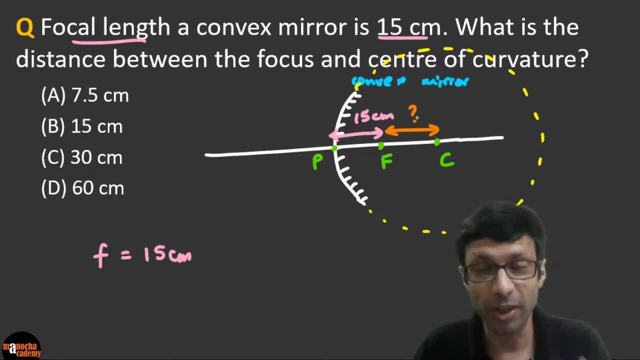 Right, CR Sharma is saying 15.. What do you guys think? So? what is the important rule here? You guys know that the focus F lies exactly between P and C, right? It lies exactly between the pole and center of curvature. Guys, you know that this distance equals this distance, right? 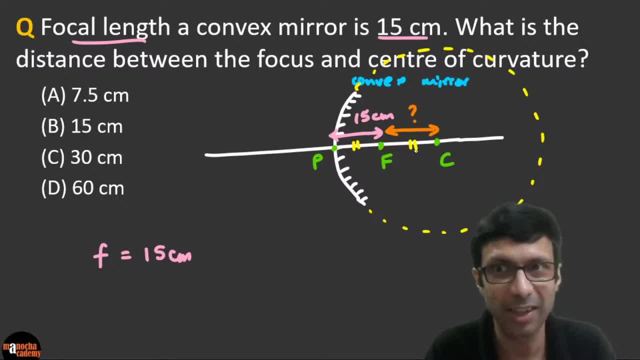 Okay. So we have not been asked radius of curvature, We have been asked the distance between F and C. So very simple answer, Because the focus lies exactly in the center of P and C. So therefore, the distance right. So we can say therefore: 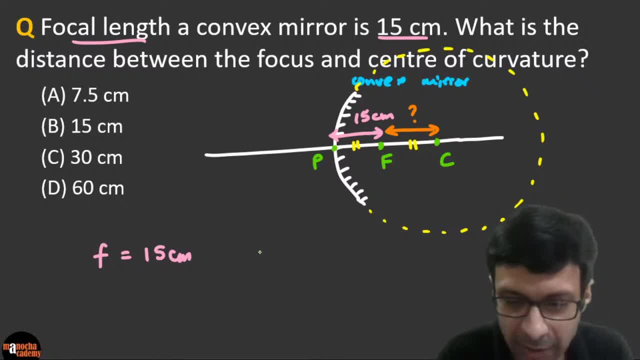 So here, guys, we can say that F- C, this distance equals P F, right, Because F is exactly in the center and P? F is the focal length, which we know is 15.. So the distance between F and C right, which we are calling as F C here, is also going to be 15.. 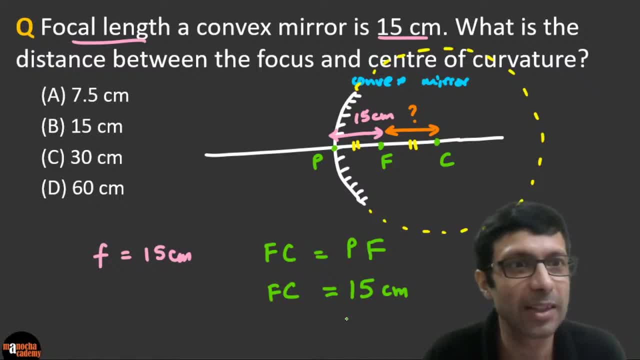 Excellent. So, guys, we have the correct answer here, Yesh has the correct answer here, Jeba has the right answer. Fantastic guys. 15.. So slightly tricky question, Don't go for You guys know this relation, Don't go for that. 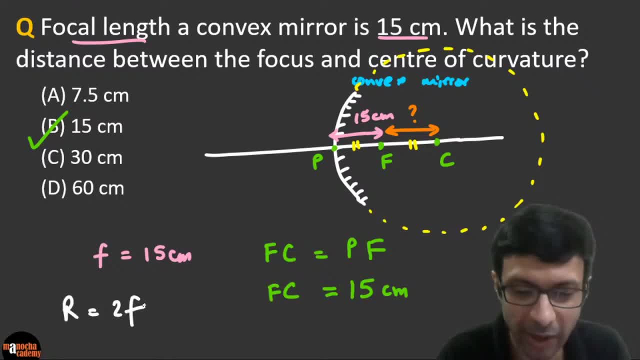 We are not talking about R equals to F, not the radius of curvature. Okay, So we are just talking of the distance F between F and C here. Excellent guys, Excellent. Next question: Which type of mirror obeys the laws of reflection? 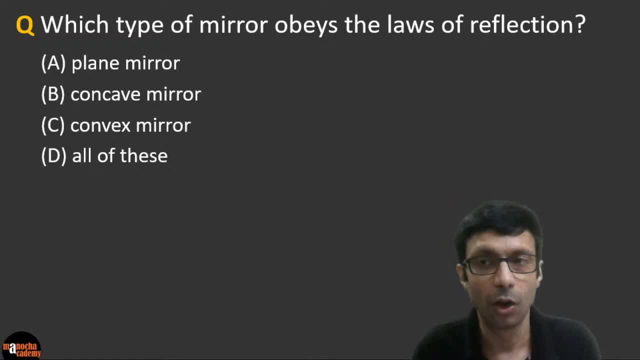 Is it the plane mirror, Concave mirror, Wave mirror, Convex mirror, Or is it all of these? So which ones obey the laws of reflection? And guys, you know, remember what are the laws of reflection. So one is that long law right. 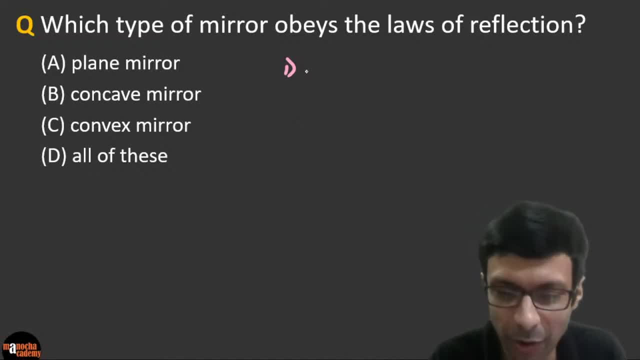 The incident ray, the reflected ray, the normal, Remember that law: The incident ray. So I don't think I'm going to write that whole thing here. Incident ray, reflected ray, right And the normal at the point of incidence. all lie, you know, at the point of incidence. 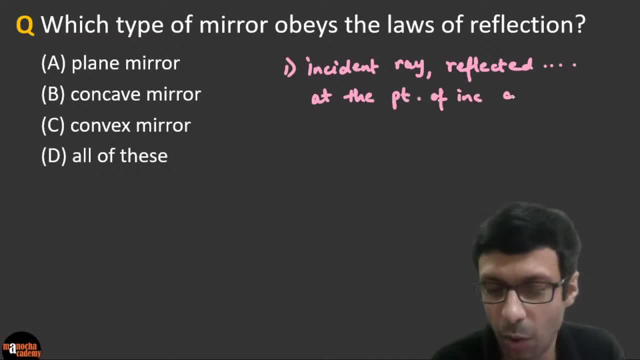 They all lie on the same plane. Remember, All lie on the same plane. So that is the first law. And what does the second law say? Law of reflection. Does anybody remember What is the second law of reflection? Angle of incidence right. 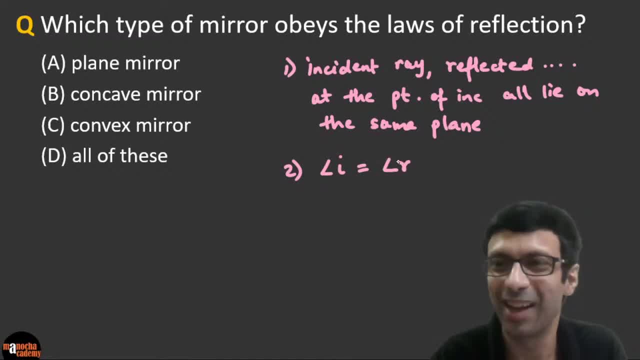 Angle of incidence equals. So this is a simple one: Angle of incidence equals angle of reflection. Now, which mirror obeys the laws of reflection? So all of you know that plane mirror obeys it, right. We know that the plane mirror obeys the laws of reflection. 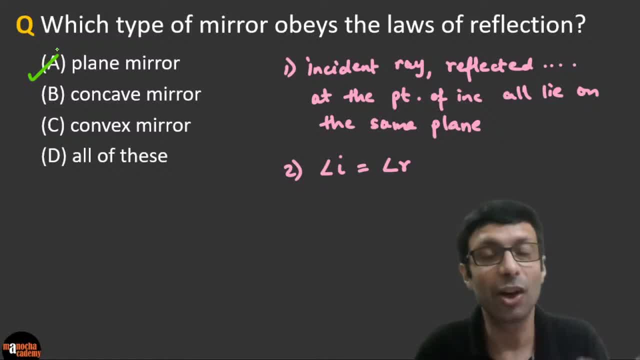 But the interesting part is that even a concave and convex mirror obey right. So whenever light falls on a concave or convex mirror, right. So let's say you take a concave mirror, whichever mirror you take right When light falls on it, right. 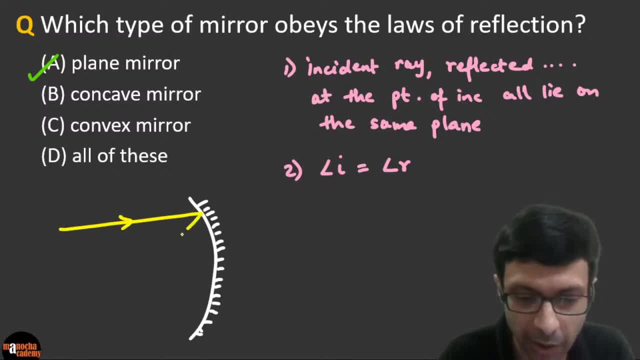 So let's say: light falls this way: Concave mirror is converging, right. So let's say: this is just a rough diagram. If that's the incident ray, this is the reflected ray, Then you can always draw the normal And you will always have angle of incidence equal to the angle of reflection. 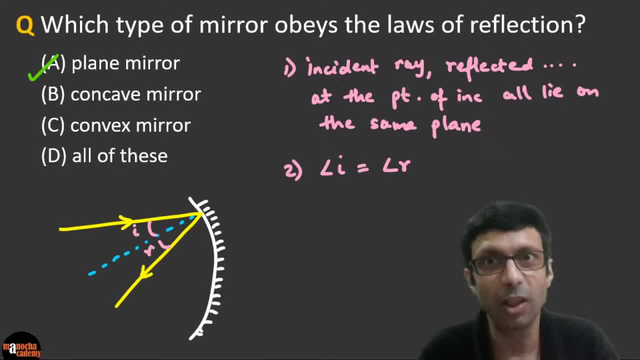 Guys, please remember this. So all the mirrors, the plane mirror, the concave, the convex, which are called, you know, the curve, the spherical mirrors. They're together known as the curve, the spherical mirrors. They all obey the laws of reflection. 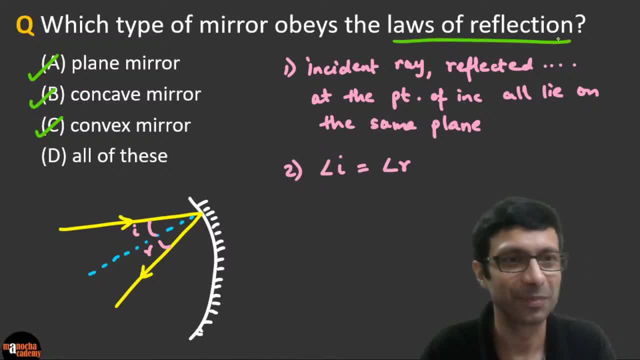 So it's not only for plane mirror. Excellent, Excellent. So I see Cecil Judson has the correct answer, Farhan Akhtar has the right answer here. Excellent, guys. So the answer will be D. All of these, because all these mirrors, whether it's plane or the spherical mirrors, the concave or convex mirror, they all obey the laws of reflection. 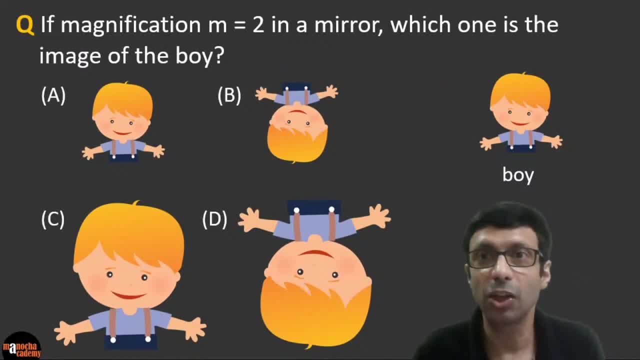 Great. Next question, guys: If the magnification is 2 in a mirror, which one of the image? which one is the image of the boy? So here's the real boy here, right Above my head. Here you can see. 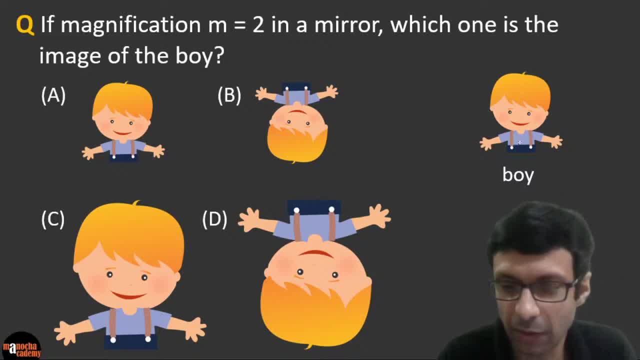 So this is the picture of the boy, Right? So can you see? This is the picture of the boy, and the boy is acting like the object here. And what is the question saying? The magnification of a mirror is given as 2.. 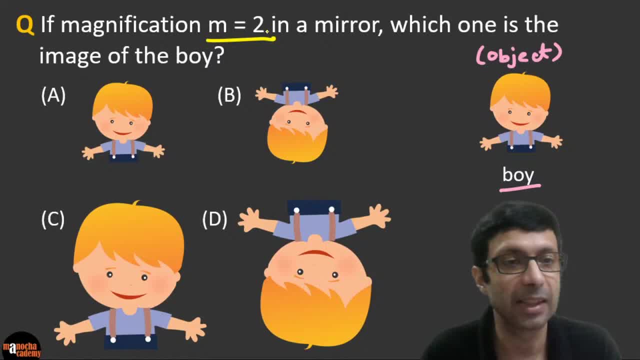 So which one do you think is going to be the image? the boy will see Which one will match. Is it going to be the picture A, the picture B, C or D? What do you guys think? And if you guys are enjoying this quiz, please hit the like button right now and do share it with your friends. 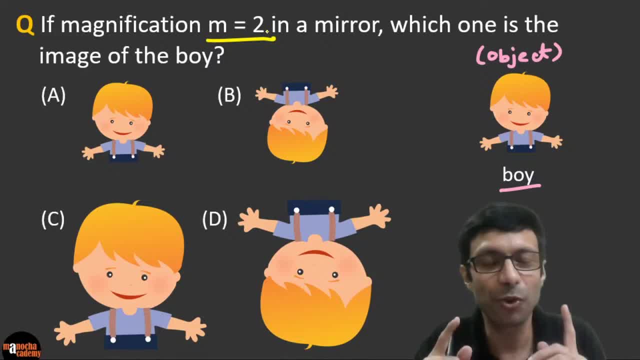 Okay. So, guys, I'd like all of you to hit the like button if you're finding this quiz useful and beneficial And please, you know, share it out with your friends. So come on, guys, Try this, Awesome, Awesome. 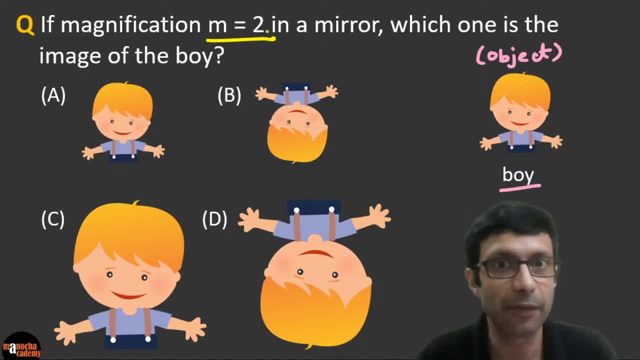 Thanks a lot. And what will be the answer here? So magnification is given as 2.. Right, So what does this number mean? Magnification, guys, you know, magnification is basically image height, which you know you can write as HI. 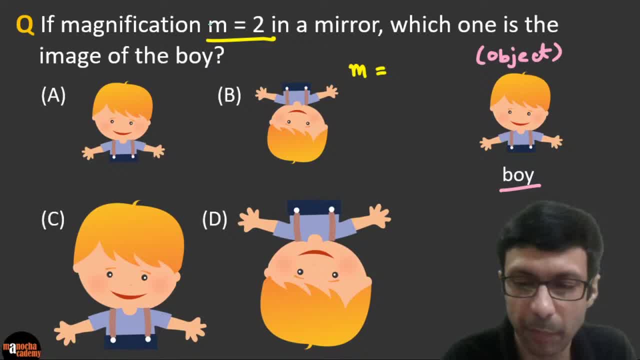 Right. So magnification, the number. magnification is basically image height divided by the object height, Or we can represent that as H dash by H, where H dash symbolizes the image height divided by the object height, H. Okay, So here you can see. we can substitute the number it's given to us as 2.. 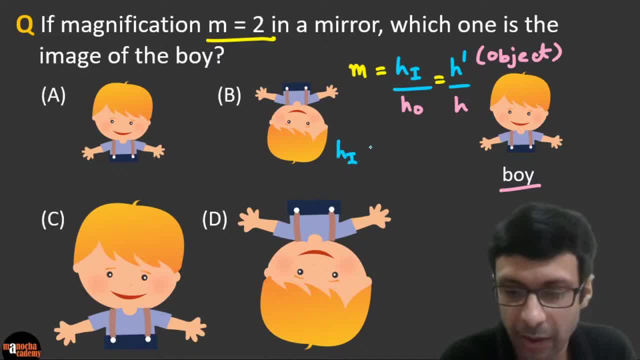 So what does this tell us? That the image height, HI, is basically 2 times the object height. HO Right, If you cross multiply, do you guys agree? Okay, So from this equation we know that the image is twice 2 times the object height. 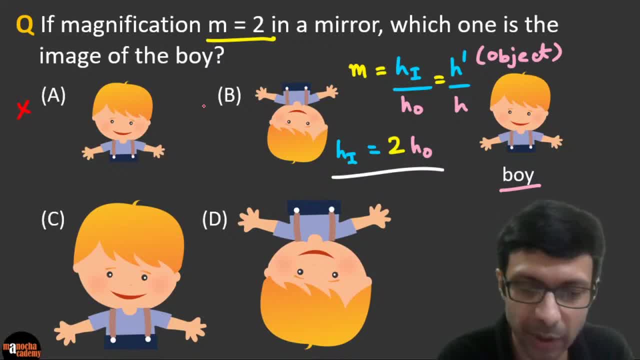 Right. So it can't be A or B Right, Because A or B is the same size. So it's not going to be this. So is it going to be C or D? So, as we'll discuss, you know, magnification has a sign if it's positive. 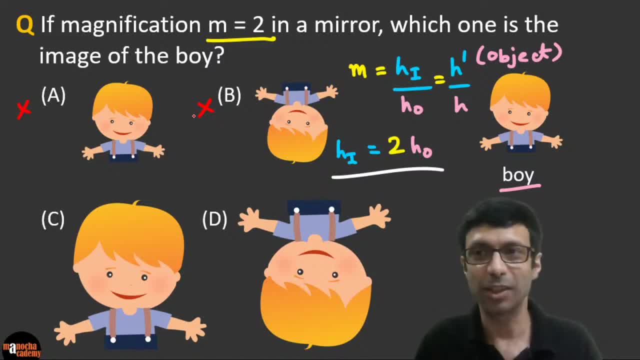 So here it's given. 2 means plus 2.. So if it's positive, that means the image will be upright Right, Because it's plus 2.. Had it been minus 2, it would have been this one, Right. 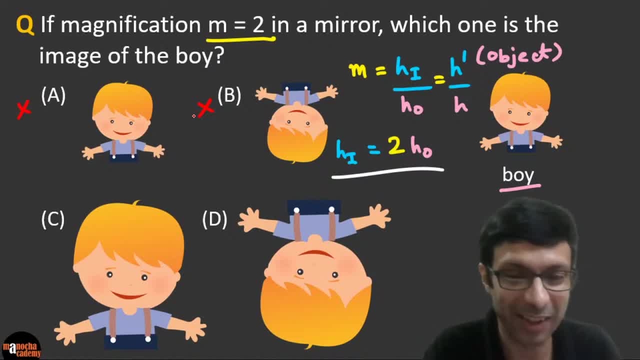 It would have been this inverted image had it been minus 2.. So the answer, the correct answer here, is C. The answer is going to be C here. Very good, I see Leena Tiwari has the right answer here, and very good. 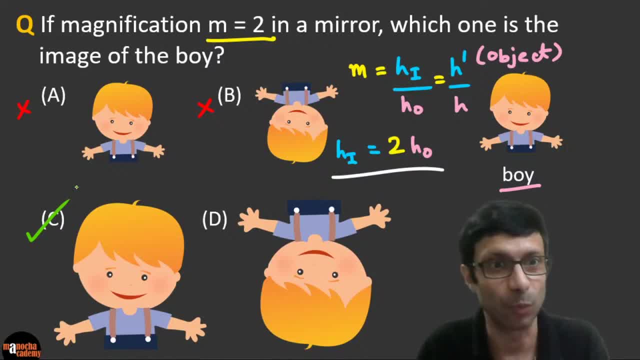 Neela has the correct answer. It's going to be C, because magnification is plus 2.. Okay, So can you see the boy is over here in this picture. The boy is upright Because minus 2 means inverted. The boy is upright and twice. 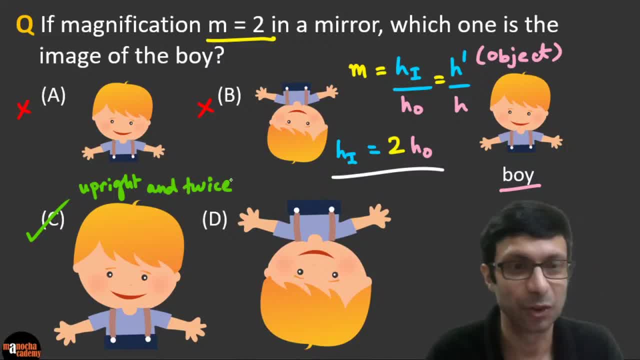 Right, The magnification is twice, So he's two times in size in the, in the height in the mirror, and it's plus 2.. So it is an upright image. Fantastic guys, Great. Let's go to our next question. Is it clear? 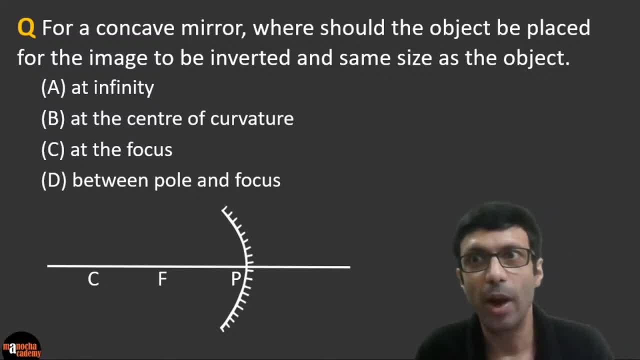 Now let's try this one For a concave mirror. where should the object be placed for the image to be inverted And same size as the object. So if you take a concave mirror here, as you can see in this picture, it's a concave mirror. 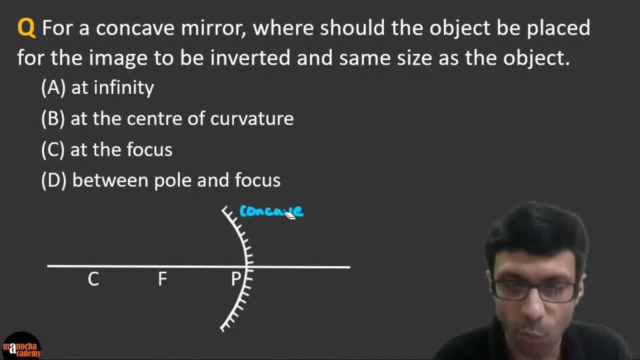 Right, So this is a concave mirror. Where should the object be placed? So where should you place the object to get an inverted and to get an image which is inverted and same size as the object? What do you guys think So? is it at infinity, center of curvature focus, or between pole and focus? 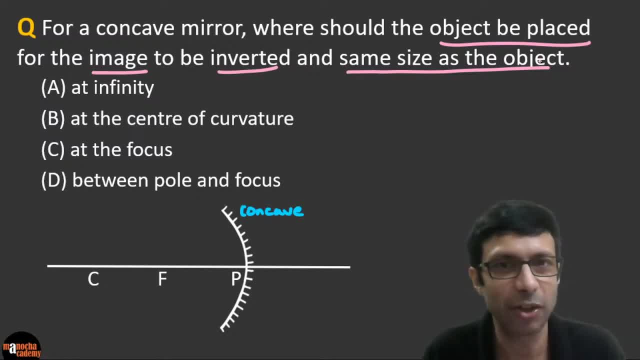 Awesome to see the participation here. Great to see that guys, Awesome. Okay, Some of you are saying center of curvature, Some of you are saying at the focus, What do you guys think? Come on, I want everybody to try here. 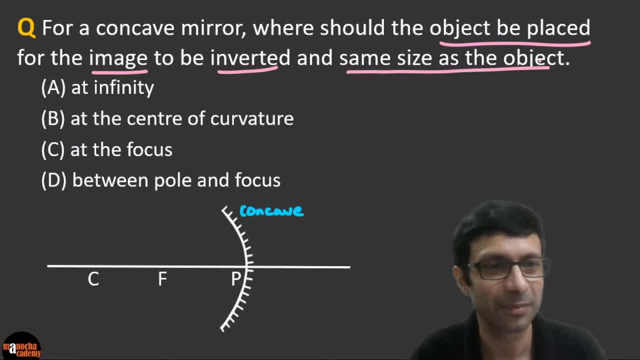 Please participate. And, guys, as I said, we have also started a Hindi classes just from yesterday on our Manocha Academy Hindi channel. So, guys, please subscribe to that Also if you're interested in classes in Hindi. it's called Manocha Academy Hindi. 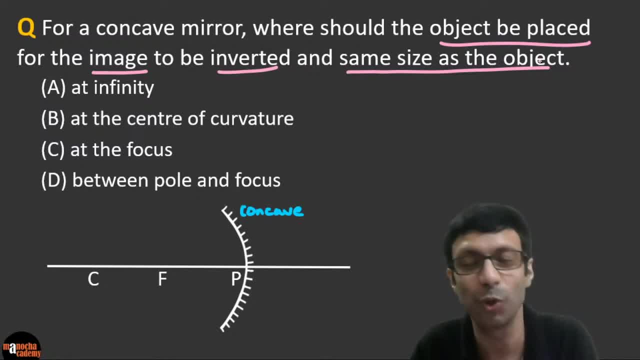 So please subscribe Manocha Academy Hindi. You can search for that on YouTube and subscribe and hit the notification bell And we'll be continuing the live classes in English here also. So both of the channels you can subscribe if you want, in both English and Hindi. 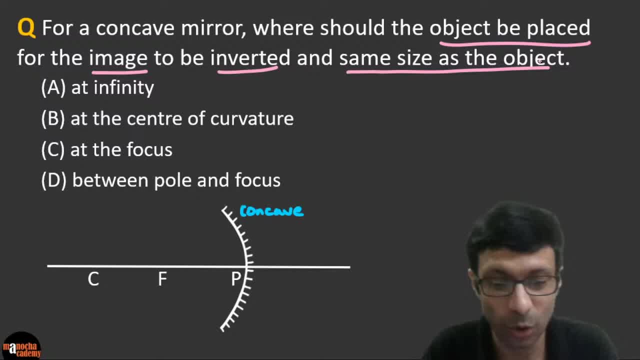 Awesome guys. So what do you think will be the answer here? So this one is that special case. right That you know that in a concave mirror here- right, This was a concave mirror If you place the object. Okay. 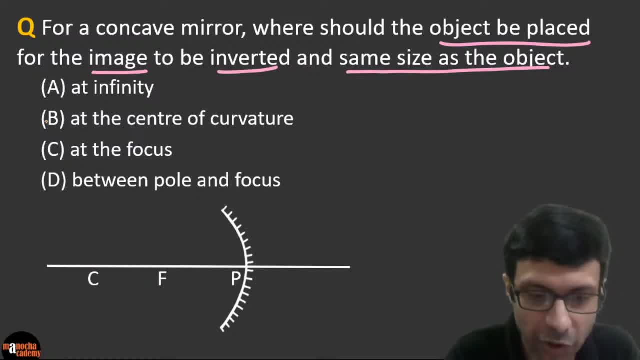 If you're going to place the object exactly at the center Of curvature. So these are our points right, C, F and P: If you place the object exactly at the center of curvature, you know that you're going to get the image, which is going to be same size but inverted. 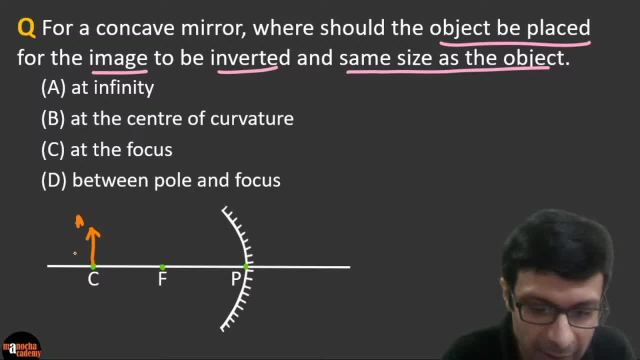 Guys, if this is the object AB, let me mark it as AB. You know the image here is going to be A dash, B dash, Same size, but inverted. Okay, So the correct answer here, guys, is at the center of curvature. 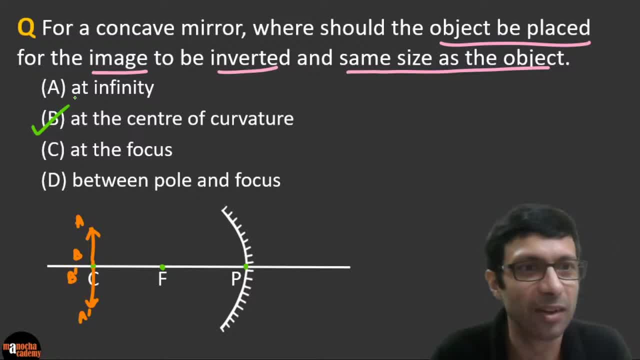 Fantastic, Very good, Right, I see Rohit has the correct answer here. B is the correct answer. Very good, Okay, So the correct answer here will be B. And guys, how to draw the ray diagram. Please practice ray diagrams. 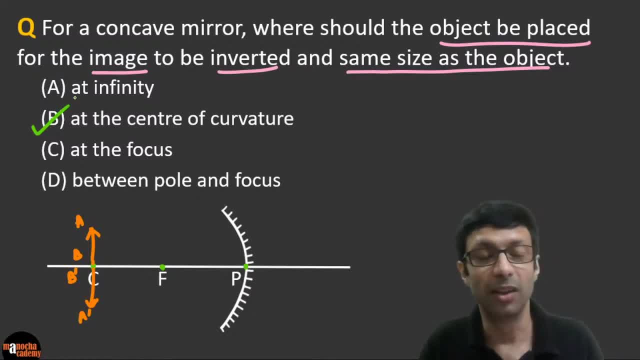 It's very important. So one is: you can, of course, use, you know the rules. For example, here you'll use a rule that you'll draw a ray parallel to the principal axis. after reflection it passes through the focus, Remember. So you can draw that rule and then you can use that rule and the ray passing through. 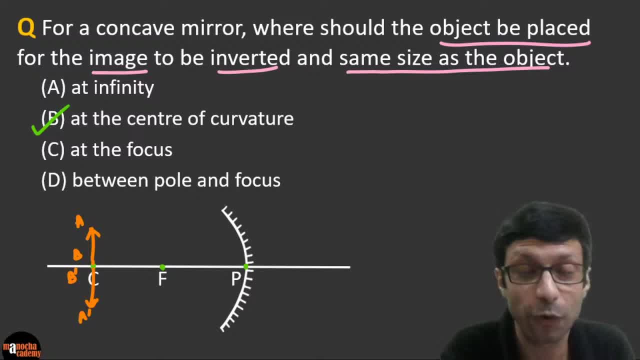 the focus after reflection will be parallel to the principal axis. But for this special diagram you can use a cheating trick right, Because you know where the image is going to be formed. for this diagram, Don't use the rules, guys, Okay. 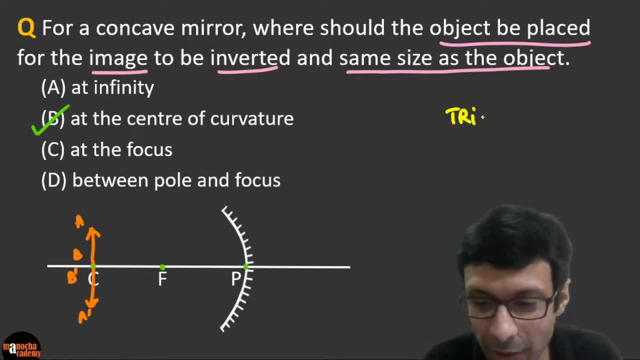 There's a nice trick I'm going to tell you. So what is the trick of drawing the ray diagram for this question? Right, How do you draw? So trick for ray diagram. So what do you guys are going to do? First, draw the image of the same size, inverted and at the center of curvature. 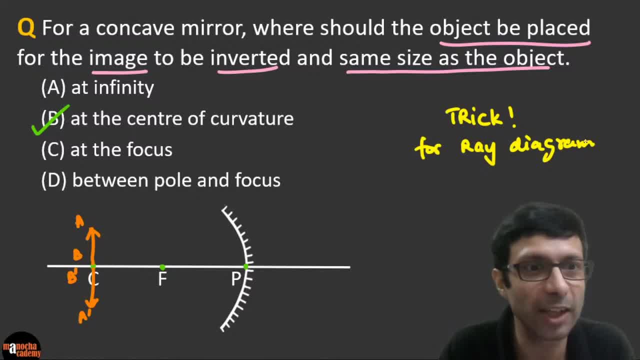 It's exactly going to be at the center of curvature. Now you guys draw the rules, draw the rays, Sorry, Okay, So don't have to use the rules Now. if you just draw the rays, you know that it's going to hit here and it's going to get reflected. 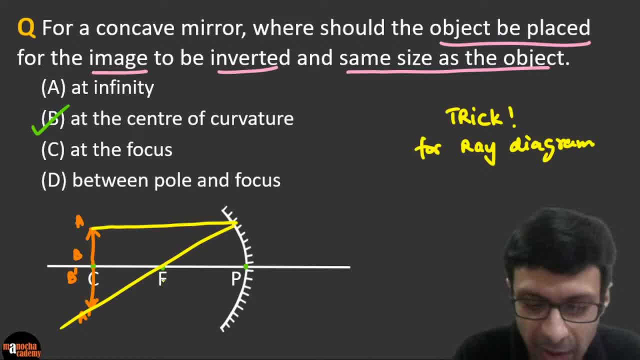 pass through the focus. Okay, And same thing here. Right, So you guys can, And don't forget to draw the arrows. You know, mark the arrows for the rays And here again you can draw. this other ray will look something like this: 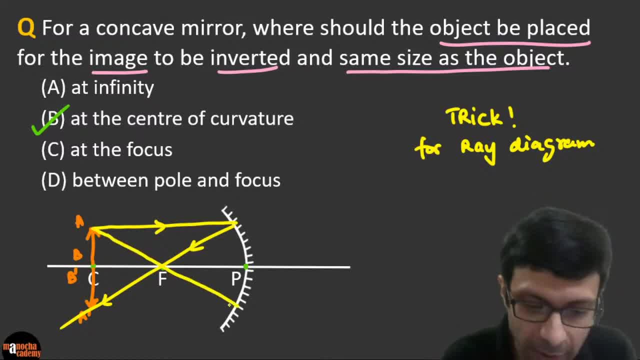 Okay, So it will pass through the focus here And after reflection it will go like this, Right? So in this you can use this trick because you know where the image is going to be formed. First draw the image, then draw the rays, because it's very hard to get it accurate. 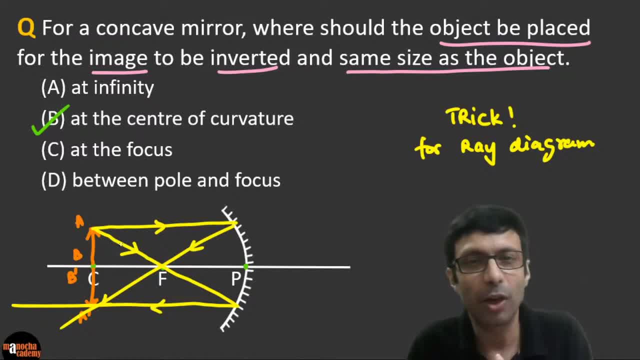 You know, if you start drawing the rays, your image may not lie exactly at the center Of curvature, And then it will be marked wrong. Okay, So here you can use this nice trick for this ray diagram. All right, guys, let's go to our next question. 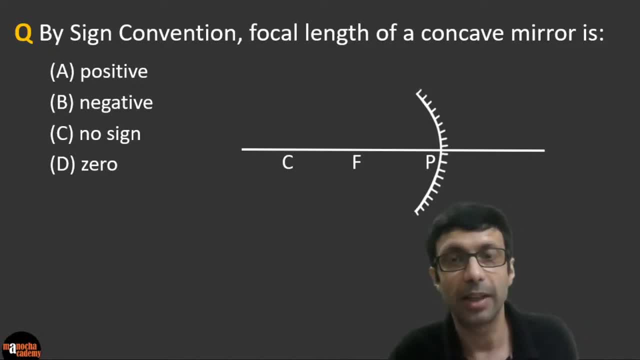 By sign convention, focal length of a concave mirror is considered to be positive, negative, no sign or zero. Come on guys, What do you guys think? And great to see 400 likes. Thank you guys. Thanks a lot. 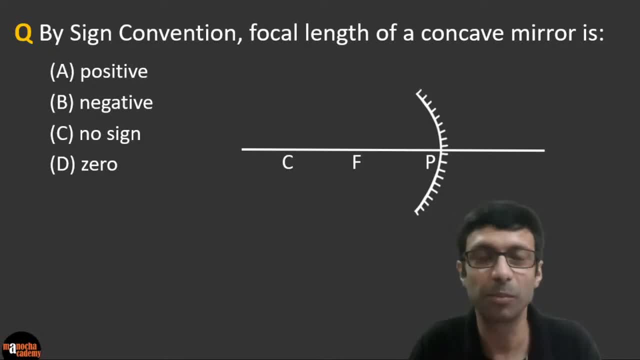 It's all due to your love and support And it's awesome to read everybody's comments. We read all the comments. We read all the comments that you guys write. So thanks a lot, guys here for your support And please try the next question. 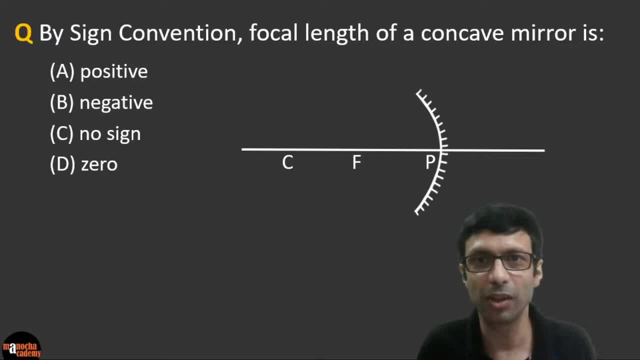 So by sign convention. So what is the sign convention? So let me teach you in a very simple way. So how do you understand the sign convention, Whether it's a concave or convex mirror? So, guys, what do you do for the sign convention? 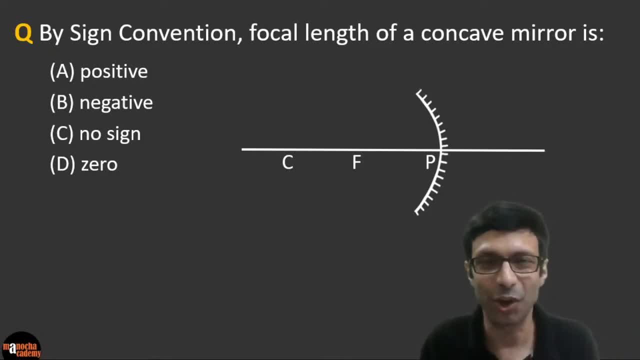 Simply draw the X and Y axis. You know coordinate geometry. If you don't know, just search for coordinate geometry in Manocha Academy, Okay, And watch my video on that. So I have a video on coordinate geometry also. So in coordinate geometry- guys, you know, you have this X and Y axis. 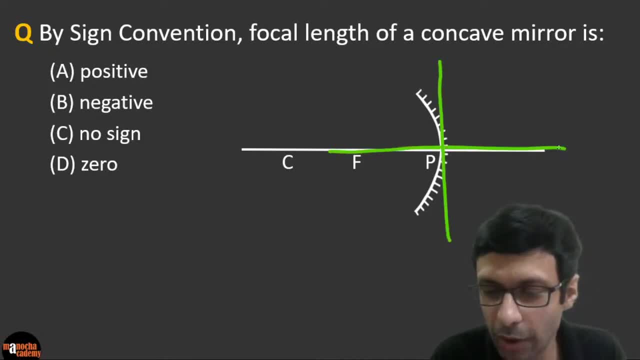 So we are going to draw them here Right. So simply draw the X axis, X X dash Right. The negative X axis. the positive Y is the positive Right. This is the positive Y axis and the negative Y dash here. 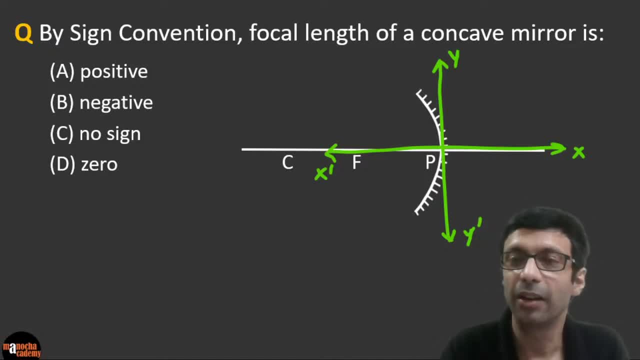 Right, Okay, Can you see that? Right, So draw these axes. One important thing is the origin. You know where these axes meet is the origin. That should coincide with the pole, Right? So can you see here, guys, the origin and pole are the same point. 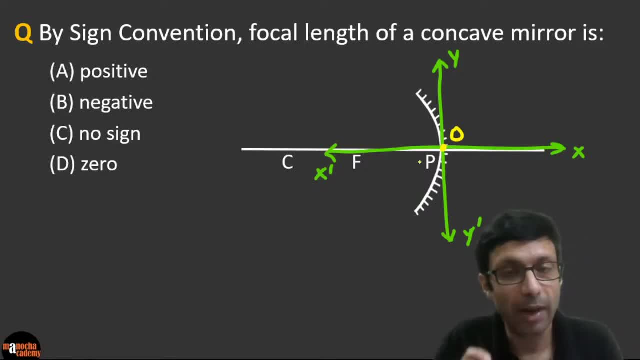 So make sure you draw your X and Y axis where the origin is exactly at the pole, whether it's a concave or convex mirror, Okay, Now what does the question say? So first you draw the axis, All right. Now the question is saying: focal length of the mirror. 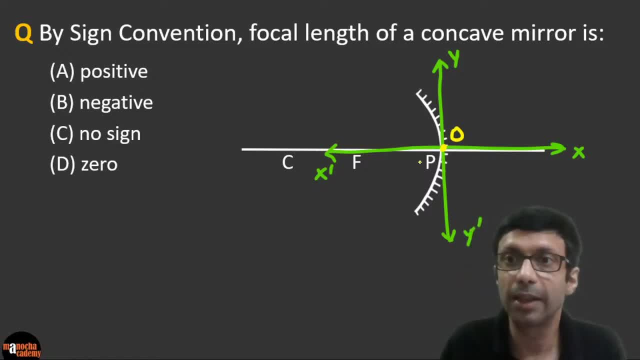 Right. So what is the definition of focal length? Focal length is the distance from the pole to the focus. You guys know this. So the distance from the pole to this focus, Do you guys agree? This is called the focal length. 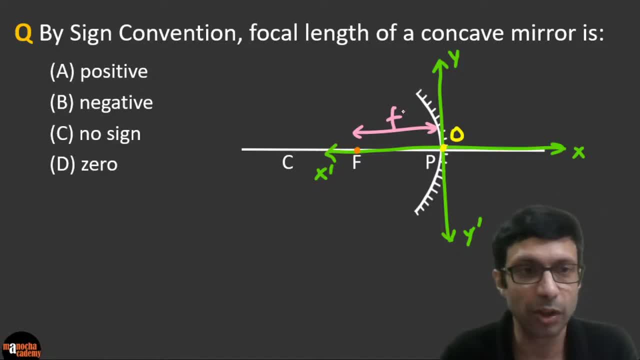 And now look at this sign convention, the axis that we've drawn, because sign convention says that, just like distances, object distance, image, distance, focal length- these all have a sign. So what will the sign be? Is it in the positive direction or the negative? 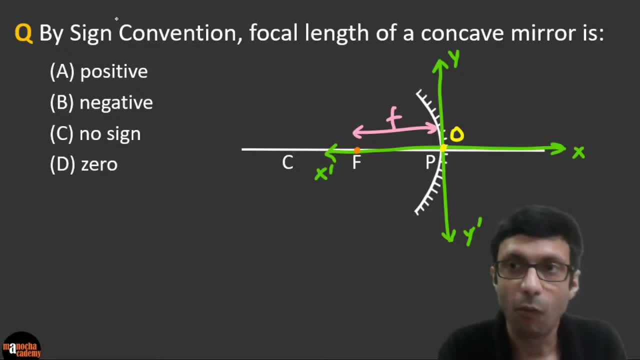 And please remember you're measuring the distance from the pole to the focus, not focus to pole. All the distances are measured from the pole. Okay, Please remember that. So I should put the arrow like this: You know, the focal distance is here, from the pole to the focus. 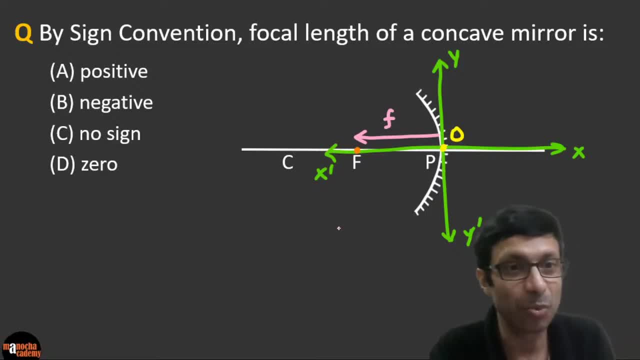 Right, So this is our focal length. And, guys, what is the focal length Right? Can you see? Very good, It's negative because, can you see, it's along the negative X axis, guys, It's along this negative direction. This is the negative direction in the X axis. 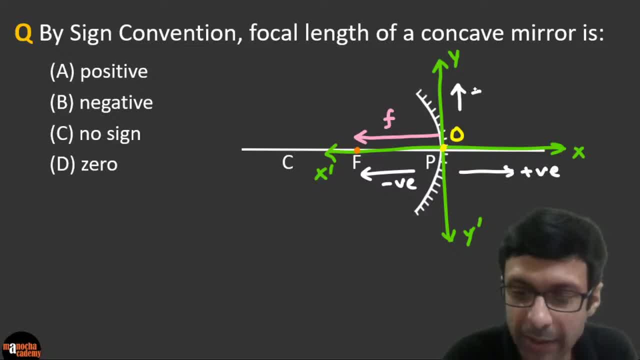 This is the positive. Similarly, Y axis also has positive, negative right. So can you guys see that the focal length from P to F is along the negative X axis? Fantastic Right. So the correct answer here is going to be B. It's going to be concave mirror always. 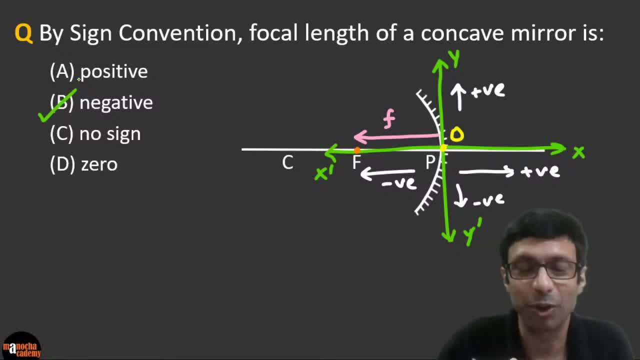 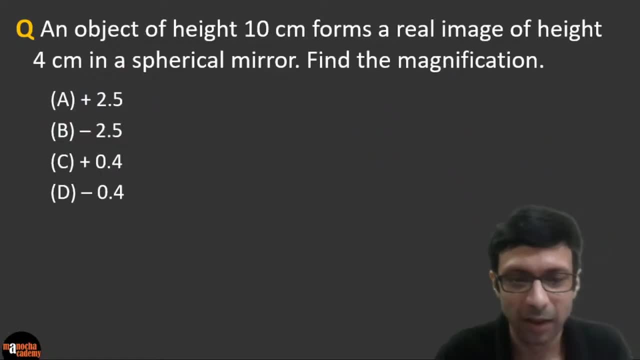 has negative focal length. Convex mirror has positive, because you know, convex mirror, the focus lies on the right side. Awesome guys. Let's go to our next question. An object of height 10 centimeters forms a real image of height 4 centimeters in a spherical. 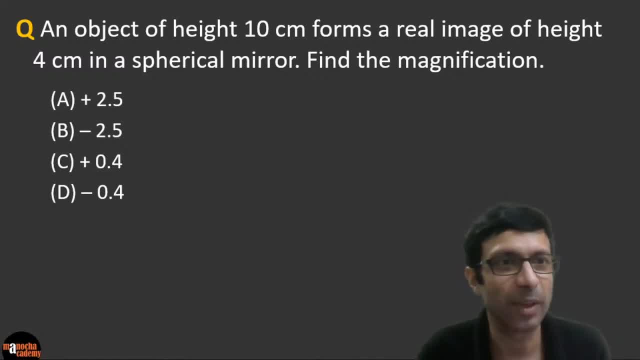 mirror, You need to calculate the magnification. So come on, guys, please try here. I want everybody to try, and sorry guys if I'm not able to take each and everyone's name here, but I'm continuously looking at the chart here and great to see your response. 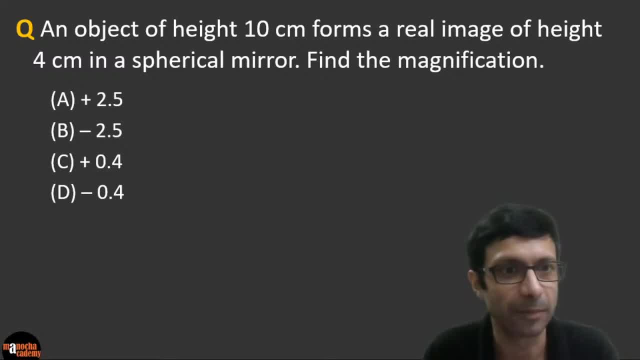 So come on. What do you think will be the answer here? Please try, Okay. Kirit says B. right, What are you guys saying? Mohammed says A. What do you guys think here? Amit is saying B. I want everybody to try here. 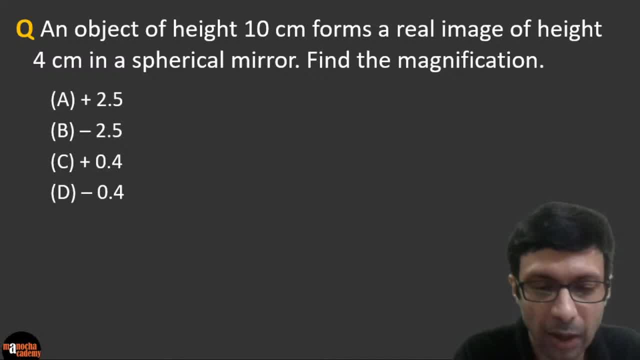 So what is the magnification? We want to find magnification and, guys, you know, magnification is a formula, Magnification, which we denote by M, just like we discussed, magnification is basically image height. Okay, Image height divided by the object height. 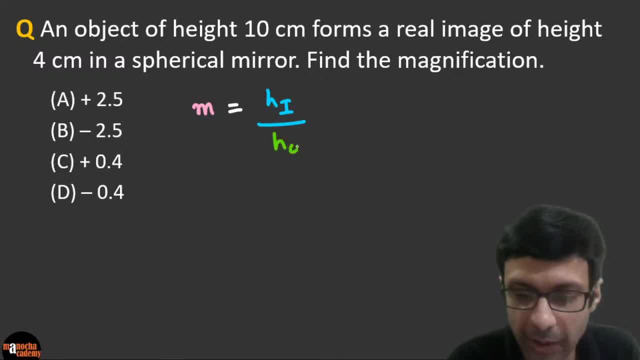 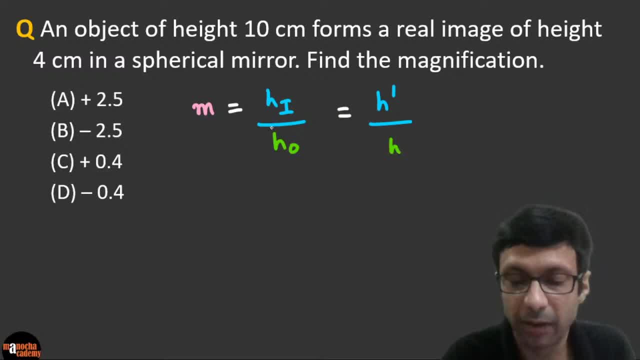 H dash by H, Where H, I or H dash. These are the image heights, The ones I have written in blue. So image height: right, So it's a ratio of the image height by the object height. Simple formula. Now please go ahead and write down the formula. 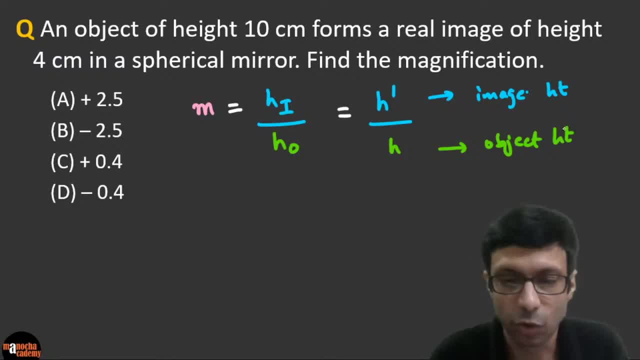 now please go ahead and write down the values. so what are the values? the object height is given to us as 10 centimeters. okay, always, guys. please write down the values, the data, clearly, so can you see: object height given to you is, sorry, 10 centimeters. right, this one an object of height, 10 centimeters, so I'll use this. 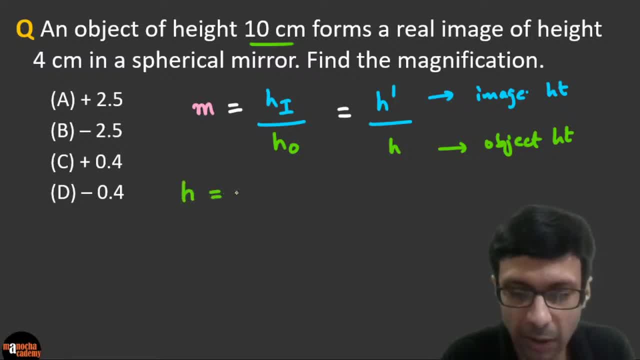 formula H dash by H. so H is given to us as 10 centimeters here. alright. and what is the image height given to us? height of the image? right, it forms a real image of height: 4 centimeters. so H dash is given to us as 4 centimeters. okay, so is. 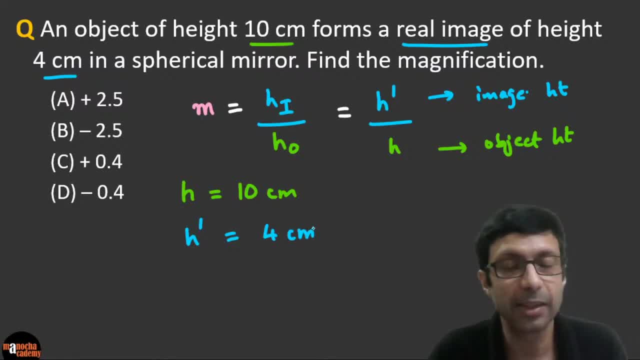 is it going to be 4? but one important thing, guys: we always have to think about the sign convention. so object, you know, is always upright. object is usually not inverted, unless given in the question. so clearly the object height is going to be just plus 10, right, or simply 10, okay? 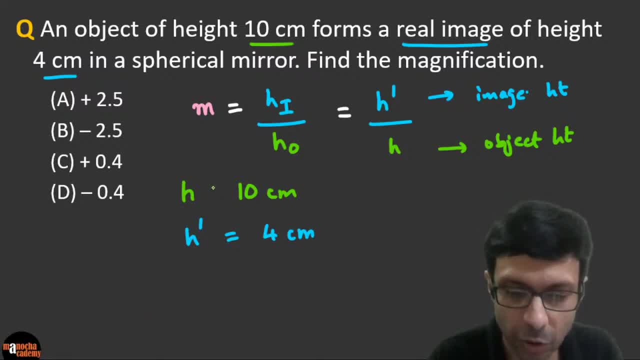 so all of you agree the object height is because object is upright. right, it is upright, so it is plus 10. but what about the image? it says a real image is formed, right. so very good, Jerry, Andy, saying the real image, right, it will be negative, right, do you guys agree? right, the real image will be negative height. why? 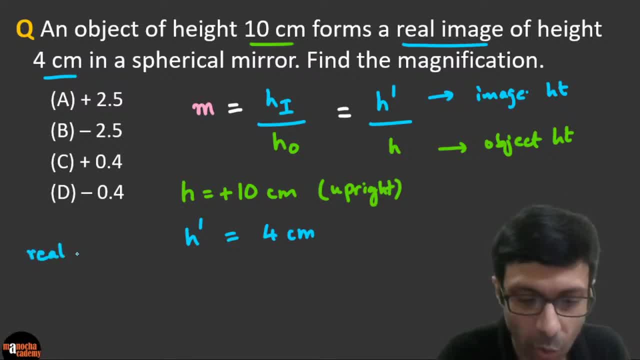 because a real image, a real image, is always inverted. real and inverted right. the image given to us is real. please read it carefully. real image is always inverted. so H dash is going to be minus 4. why? because it is an inverted image. why is it inverted? because it's a real image. real image is always inverted. 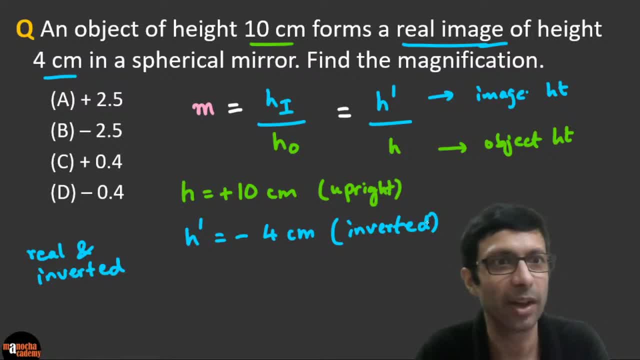 now use this formula and see what do you guys get. okay, so Anil Mishra is getting minus 0.4. what are you guys getting? so come on, all of you, please try. so M equals H, dash by H, H dash by H, and you just need to substitute these values, right, and so what? 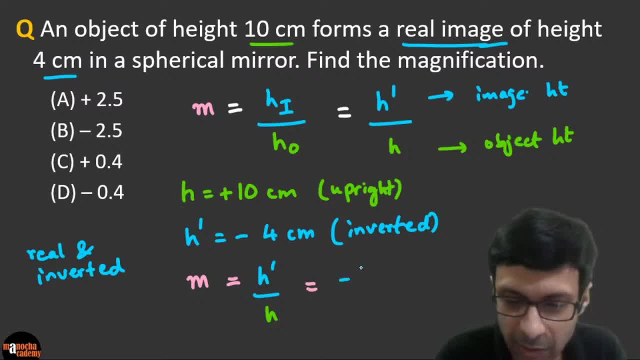 is that going to be so? H dash is minus 4 centimeters. minus 4 centimeters divided by plus 10 centimeters. okay, and guys, the units will cancel right, it's, the unit simply cancel off and you're getting minus 4 by 10. please check my. 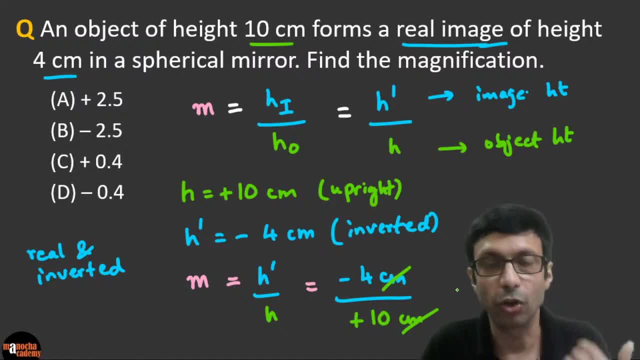 calculation right. so have I done the right thing here? please check, because object is always upright. so it's positive in height. image is a real image. it's given to us. it's negative in height- excellent, I see Pragati also has minus 0.4. very good, okay, all of you are. 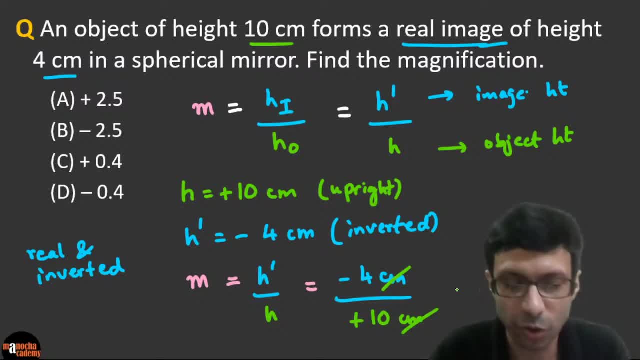 getting the right answer right. Sanya Sheikh also has very good, so the answer is going to be minus 0.4 here. excellent, because it is M equals 4 minus 4 by 10, so our answer is minus 0.4, right? this is the magnification, clear. 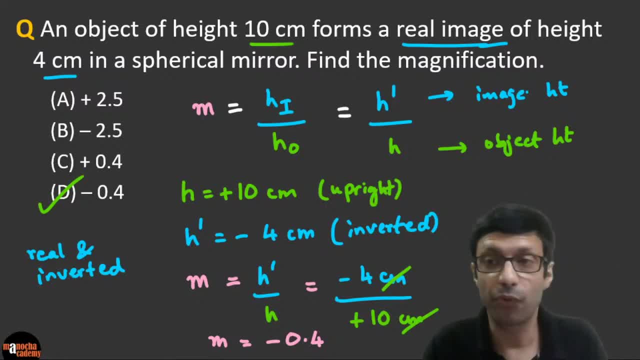 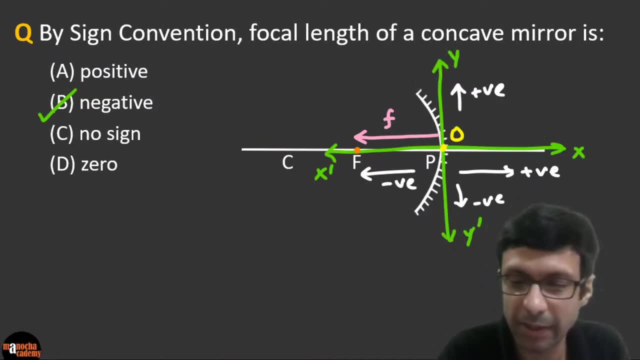 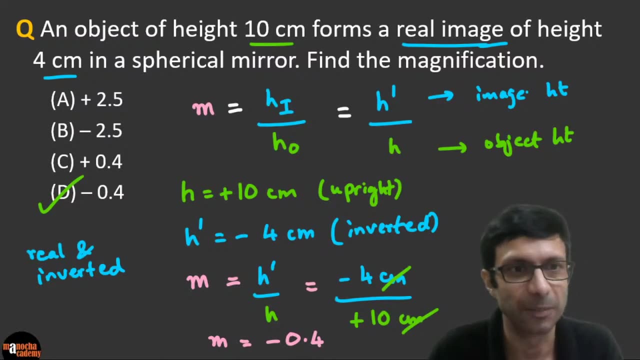 let's go to our next question. so please, guys, don't forget the sign convention, very, very important, and it can be used for the distances as well as the heights here. so here we are basically using the y-axis right. anything upright is positive, this inverted is negative. that's why we did this here, awesome. 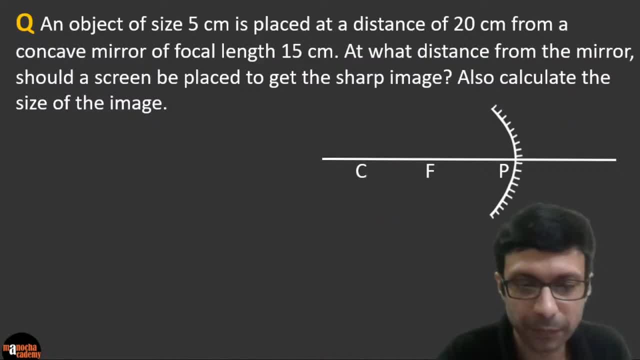 awesome guys, great going, and let's try our next question here. so what does this say? an object of size 5 centimeters is placed at a distance of 20 centimeters from a concave mirror- okay, of focal length 15 centimeters, so it's a slightly 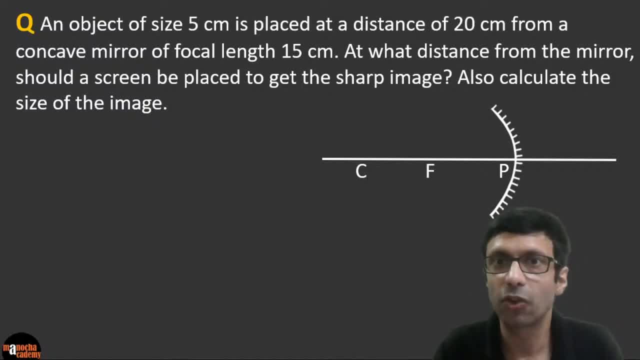 long question: at what distance from the mirror should a screen be placed to get to get the sharp image? also calculate the size of the image. so come on, I want all of you to try. let's make it. I'm going to make this complicated question really simple for you, okay. so how do you make it simple? first of all, please draw. 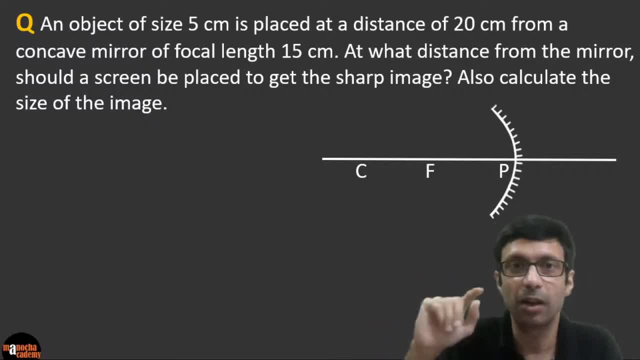 a diagram, okay, so I've got this picture here of the concave mirror. you need to sketch this rough diagram. it's very important, all right. so please draw this diagram first and let's see what we can do here. so we have been given an object of size 5 centimeter, all right is placed at a distance of 20. 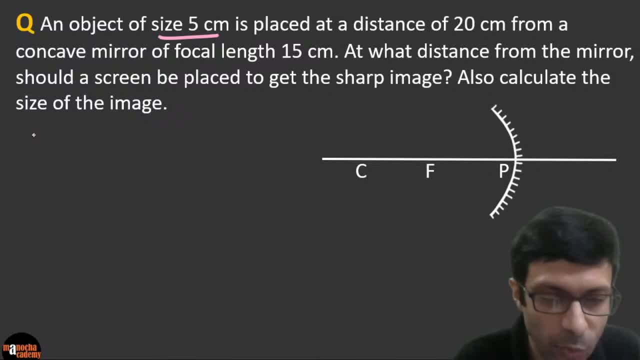 centimeters, right? so object of size 5 centimeters. so let's quickly write that down. so that means the object height H is 5. always think is it going to be plus 5 or minus 5? object is always upright, right? okay, so we can say that the object height will be plus 5 centimeters. 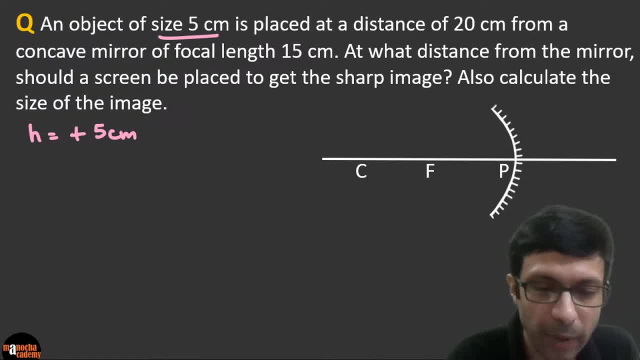 and also let us draw the rough diagram right. so let us place our object here. so it is placed at a distance of 20 centimeters, so it is placed, you know, somewhere here, right, because the focal length given to us is 15 centimeters, okay, so, guys, you can see here the focal length, which is this distance. 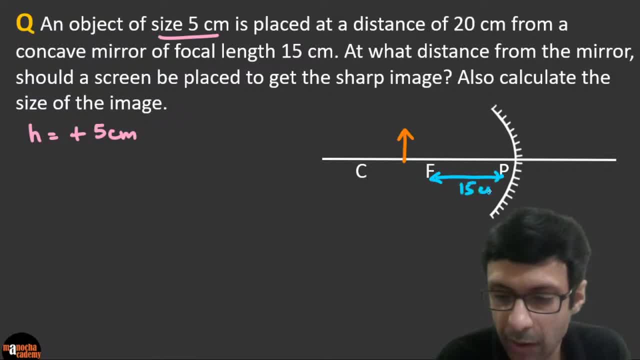 from p to f is given to us as 15, and the object is placed at distance of 20 centimeters from the mirror. so this is 20, okay. so let us write down that thing, let us write down the data and please do not forget the sign convention. okay. so, guys, remember. you know you need to draw your axis here. 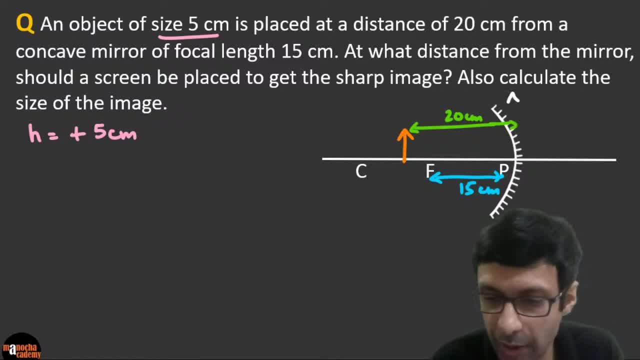 this is going to be the axis, or let me use: you know a different color here for the axis. so what is our axis going to look like here? okay, so we have these axes here, right? all right, so that's our x, x dash, y, y dash, right? oops, i'm hiding the y dash there. can you guys see? 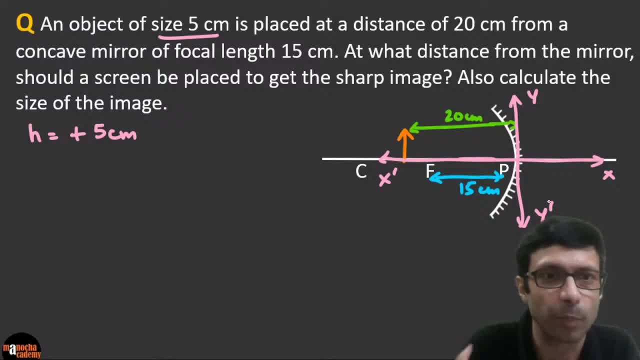 so please draw the axis and work with that. okay, so please work with the uh, with these axes for your sign convention. so h is clearly on the positive y axis, so h is plus 5 centimeters the object height. okay, so let us draw the axis and work with that. okay, so let us draw the axis and. 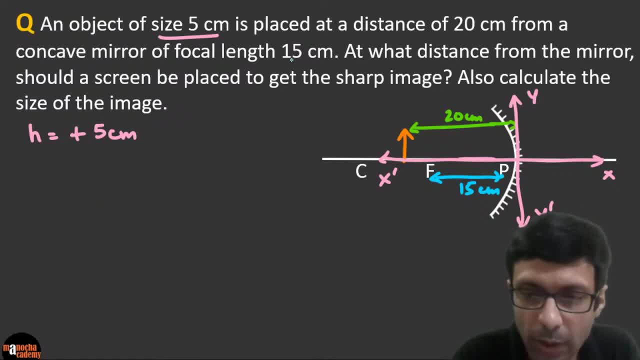 what is the focal length going to be, guys? so focal length is given to us as 15 centimeters. so please write down the data. so is it positive or negative? so f is 15, but you can see that the focal length is along the negative x-axis. can you see? it's along the negative x-axis. so the focal 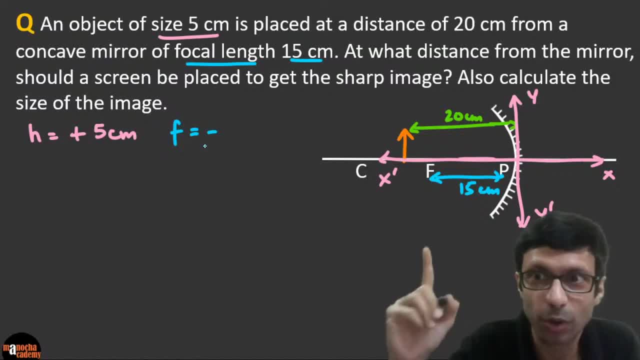 length, guys, is going to be. what is it going to be here? please note, it's along the negative x-axis minus 15 centimeters. okay, and what about the object distance? so object distance given to us is 20 centimeters, right, okay. so h is the symbolizes, the object height, f is the focal length, right? 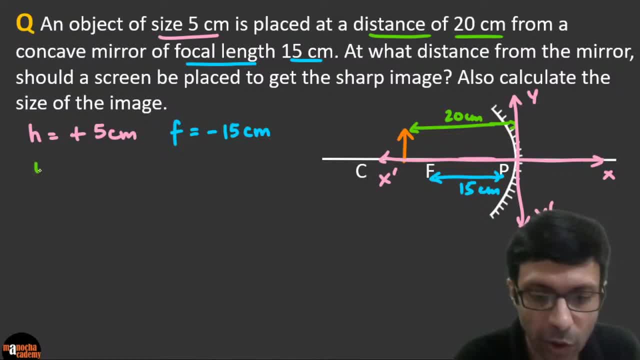 and here we have been given the object distance which we call is as u: okay, u is the symbol used here, so u is going to be minus 20 again, because can you guys see that it's along the negative x axis from p to the object? okay, very good. so minus 20 centimeters, all of you. clear about this thing. 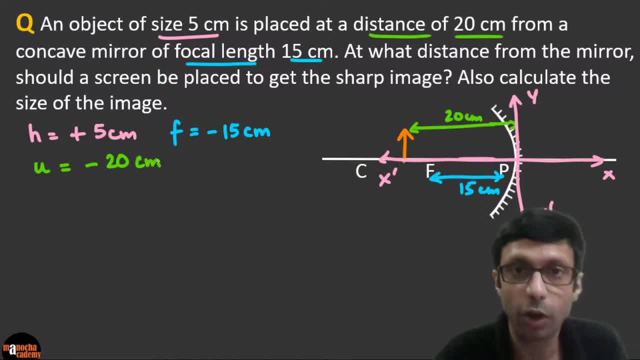 we are using the sign convention here. so for all your data that you are writing for these sums, okay, we need to write down the this data with the correct sign. of course, you can solve this question by ray diagram, but usually we will go for the mirror formula. we are not solving it using ray diagram. we are going to solve 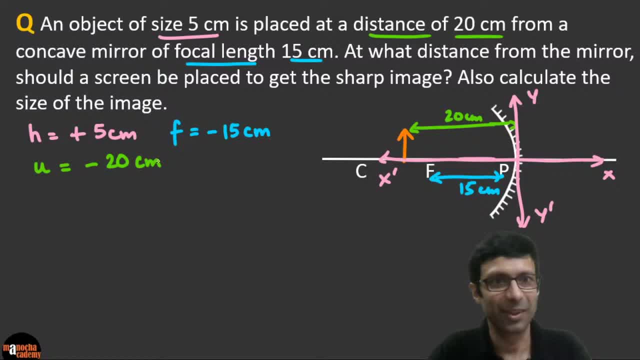 this question using the mirror formula. okay, so let's go ahead and use. do you guys know what is the mirror formula? we have written this data. and one more thing: we need to find at what distance from the mirror the screen should be placed to get a sharp image. that means we want to find the 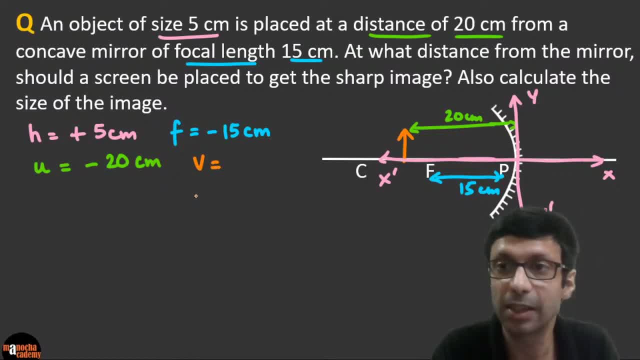 image distance. so let's call that v and for image distance, since it is unknown, we don't have to take the sign. we are just going to put a question mark, okay? so what is the mirror formula, guys? so you don't have to draw a ray diagram, just draw this rough. 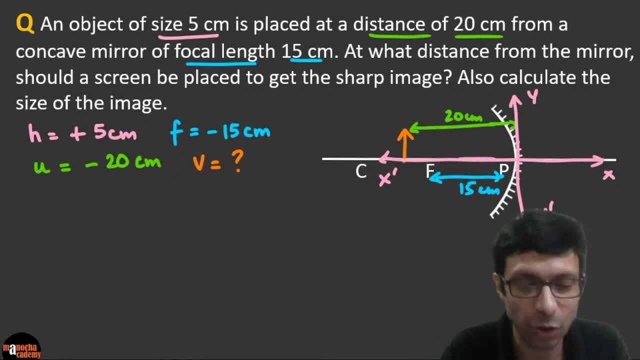 diagram and we are going to do it with the mirror formula. so you guys know what is the mirror formula. it's basically 1 by f, right? have you seen this mirror formula? 1 by f equals 1 by v plus 1 by u. this is called the mirror formula. all right, okay, so go ahead and use this formula and please. 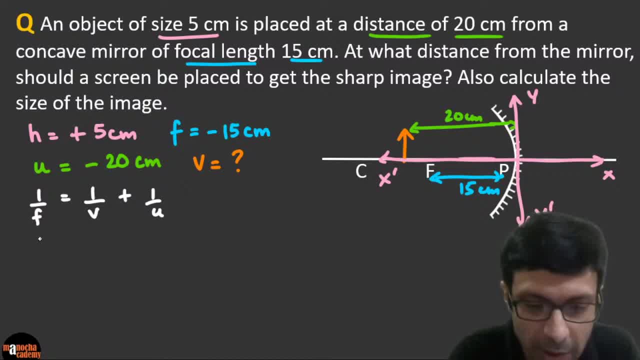 substitute the values here and work it out, right. what will it be? basically going to be 1 by minus 15, because focal length is minus 15 v we need to find. so that's going to be 1 by v and plus this is going to be 1 by minus 20, right, because u is to a minus 20 here. 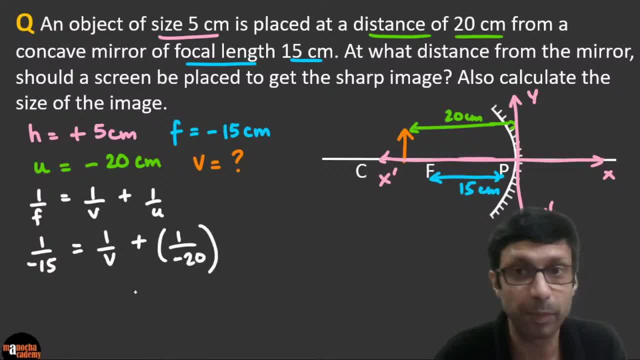 so please substitute with the correct sign. so i'm getting this. please check right in case i'm making any mistake here, because i'm also solving it live here, so go ahead. very good, i see, tanish has written the correct formula. so this is called the mirror formula, guys. 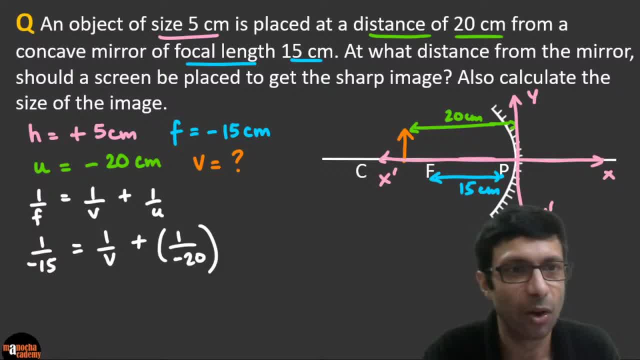 okay. so now i want all of you to calculate this and try. so come on, guys, please try. awesome to see the response. excellent, guys, okay. so please go ahead and try this question. and what do we get here? so basically, we will get that you have 1 by v. so how do you solve this? you bring 1 by v on this side and basically we are getting. 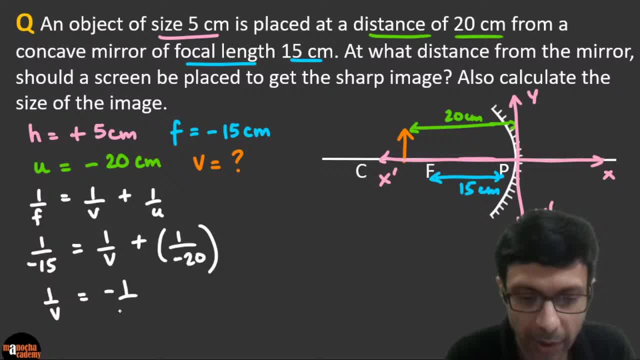 minus 1 by 15, right? so 1 by v is minus 20, right? so we are getting minus 1 by 15, and so we are getting is going to be minus 1 by 15, plus 1 by 20, right, because if you move it to the other side, you will. 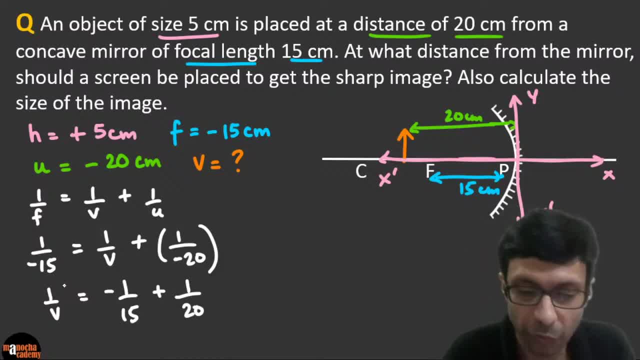 get a plus there, right, and so if you guys solve this, what will you get here? please calculate it so you just have to take the lcm. so the lcm is going to be 60 here. this is going to be basically minus 4 plus 3- is what i'm getting right- 1 by v. so therefore we are getting 1 by v equals. 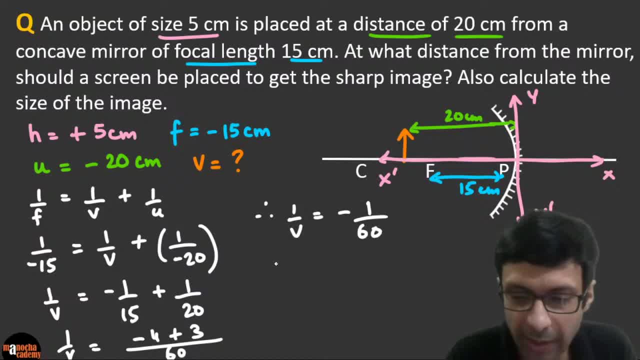 minus 1 by 60. so what is v, guys? or? v equals minus 60 centimeters. are you guys getting this? please check? awesome, i see. jude has the right answer. binod has the right answer. excellent, minus 60. don't forget the units. physics units are very important. centimeters, can you see? i've 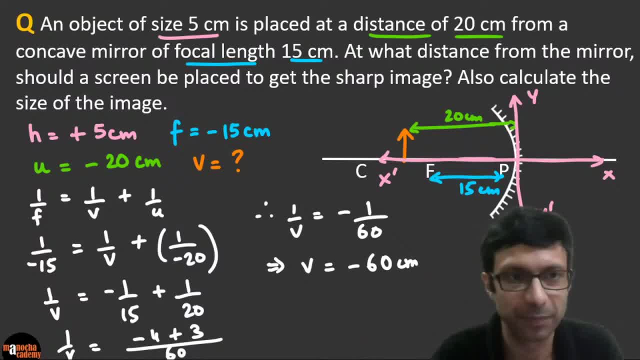 written here: minus 60 centimeters. okay, so that is v our image distance. guys, we have found the image distance using our mirror formula. here, 1 by f equals 1 by v plus 1 by u. you didn't have to draw a ray diagram, clear, so this is the answer. now, what is the meaning of minus 60 centimeters? okay? 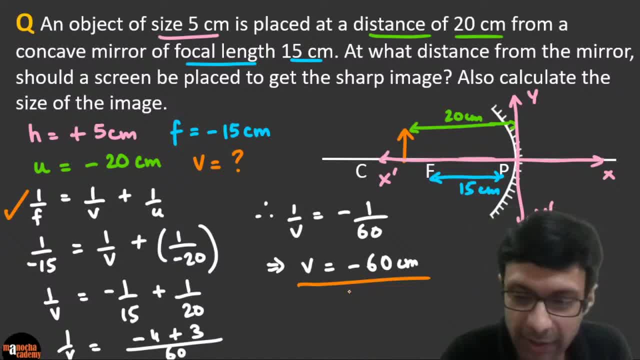 so you can write it. so you can write this down. you've been given minus 60 centimeters. that means: is it in front of the mirror or behind the mirror? so we can write it in a sentence form: right? so this means image is formed right, 60 centimeters. will it be in front or behind, guys? because minus 60 that means clearly the image. 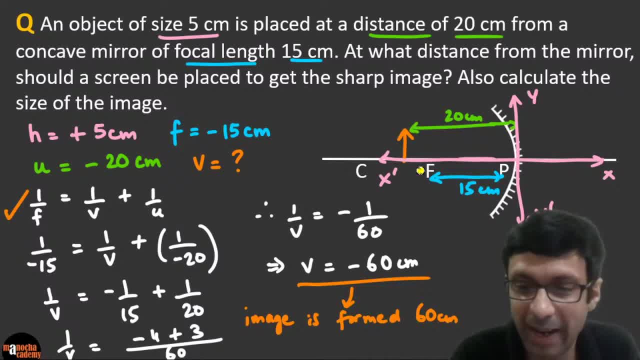 is going to be formed this side, right along the negative x-axis. that means in front of the mirror. all right, so it's going to be formed 60 centimeters in front of the mirror. right? that is our answer, so you can write it also. please write it in sentence form, right, because that we are. 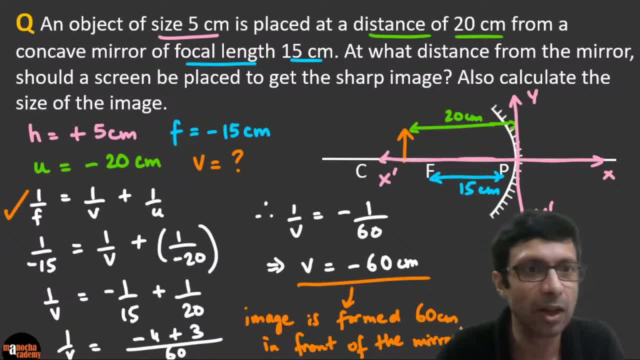 analyzing. so, rather than writing left, very good. some of you are saying left. don't say left here. say in front of the mirror and right will be behind the mirror if it was formed on the right. do you guys agree? so, yes, very good. i see sri har is saying in front of the mirror. 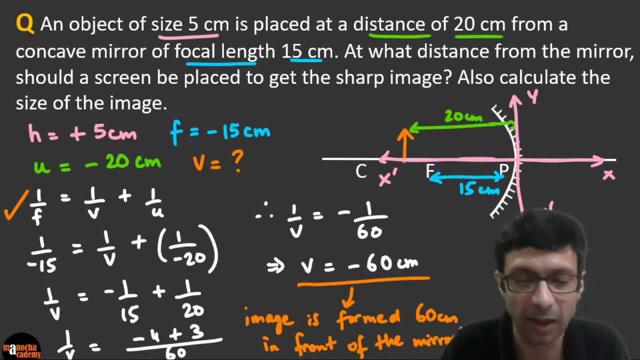 excellent. so much, paul also says that. very good, guys. and what is the last part left? also calculate the size of the image. so is this crystal clear, guys? so just you know, write down the data with the correct sign, write down the mirror formula, substitute, and it's so easy, and, guys, 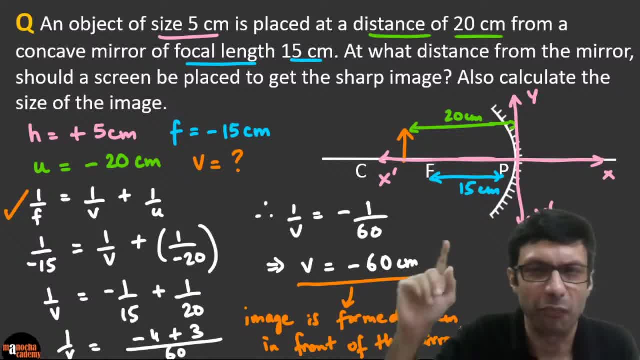 please make sure you draw this diagram. very, very important to draw a rough diagram without any rays. why? because we are using mirror formula. so draw a rough diagram. mark the rough data there. draw the x and y axis, as i have shown you here. right this coordinate axis very important, which. 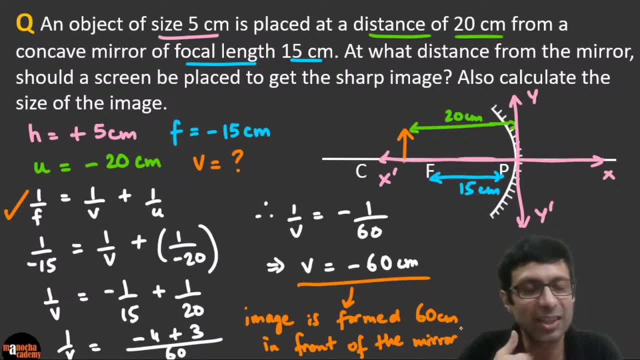 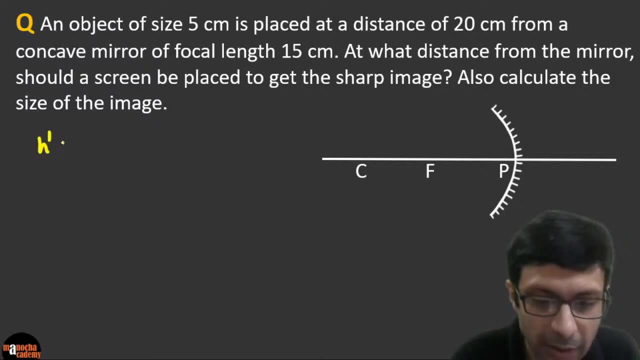 is centered at the pole. decide your signs based on that. just substitute and solve. very simple, okay. and the last part? let's do that on our next slide. we need to find the size of the image, okay. so size of the image means we need to calculate what is h? dash, right, we are interested in the size of the. 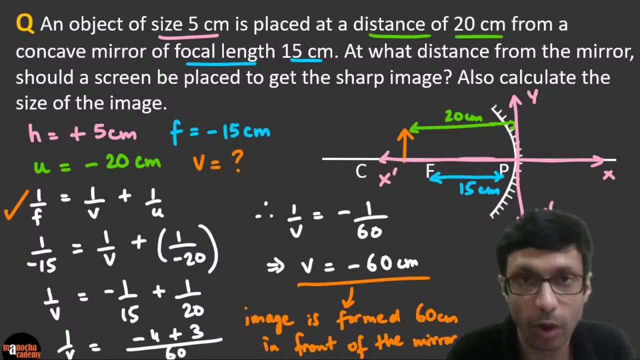 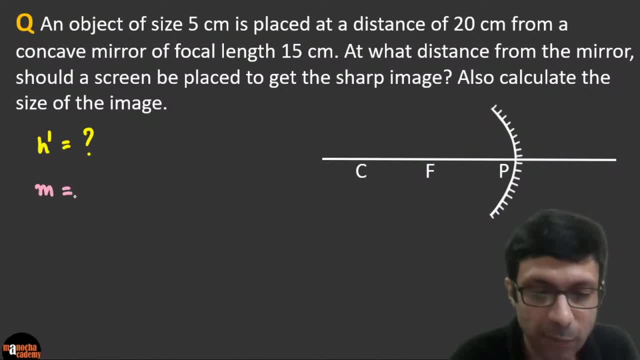 image, here, h dash for the same question. now, what is the important formula? we are going to use the magnification formula, guys. magnification, you know, as we have discussed, magnification is basically h dash by h, the image height by object height. but that's also, guys, that is also. 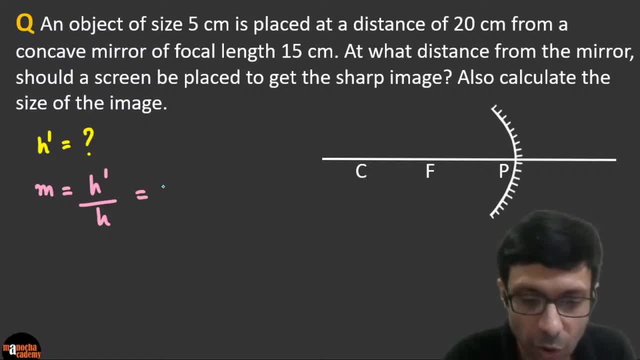 equal to minus v by u. right, it's also equal to minus v by u. very important: there's a connection between the magnification, the h dash by h, and the image and object distance. v is the image distance, this is not velocity. right, v is image distance, u is object distance. so, guys, please use this formula. 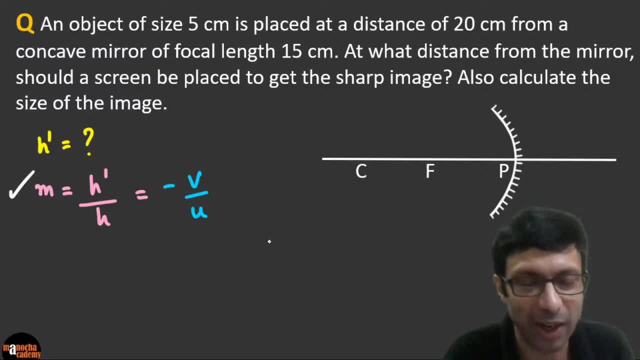 and we can easily find out the image height. why? because we know the object height. you saw, we have written previously: object height was plus 5 centimeters, so we know everything. h is plus 5 centimeters. the object distance was given to us. can you see? object is 20 centimeters in front, so u was minus 20. 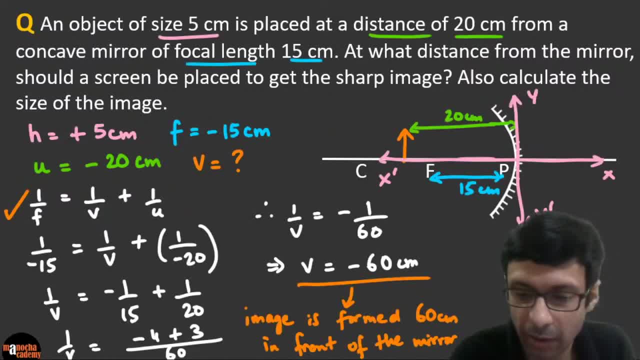 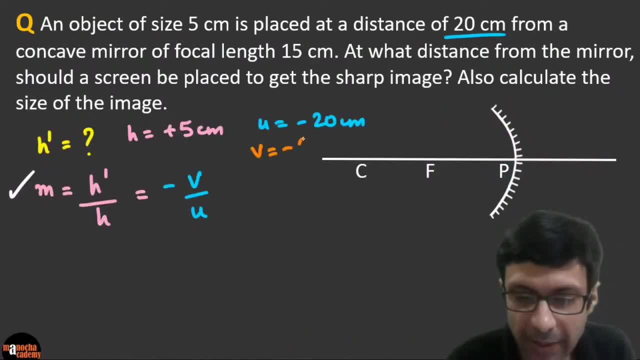 with the correct sign. and what is v? we have calculated v. v is right, so v is minus 60. right, as we calculated v was minus 60 centimeters here. so now we just have to substitute this in this formula, right? so we are going to get. 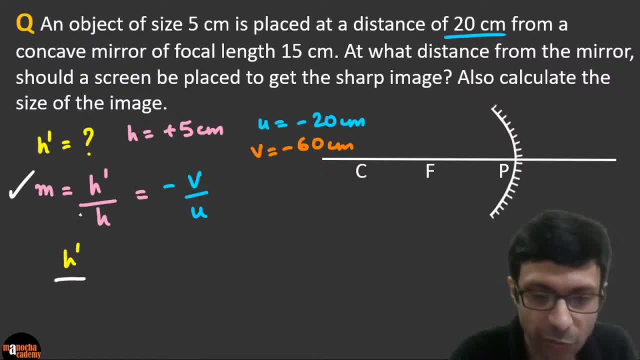 h dash by. divided by h is 5, right, so 5, and that equals- don't forget the minus sign- minus v by u, so minus v, so v is minus 60 here. so we are going to plug in minus 60 for v. okay, and divided by: 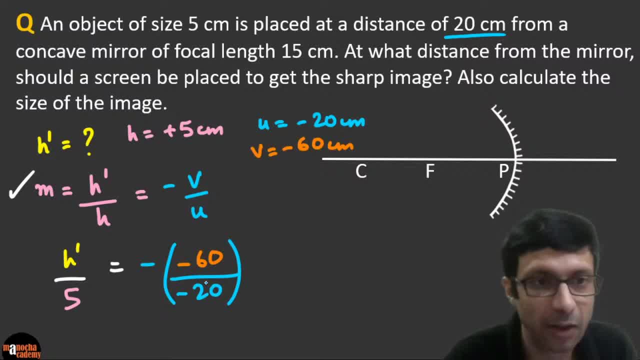 u is minus 20.. do you guys agree? so please don't forget the sign here. please check it. okay. so minus v by u. right, and now go ahead and uh, use these values here. so h dash by h equals minus v by u and basically this minus sign will cancel our frame and this will also get cancelled. 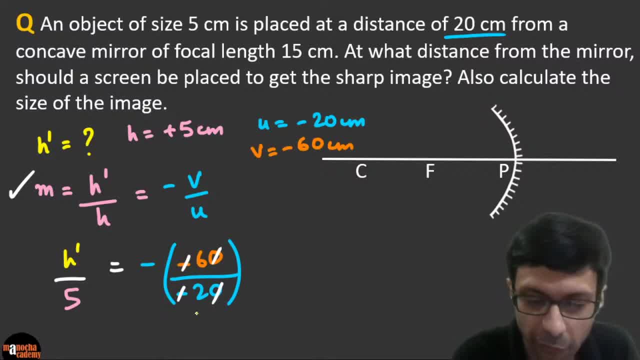 the zero. so we are basically going to get h dash by 5. right, so we get h dash by 5 is minus 3.5.. are you guys getting that? please check my calculations in case you know i make some mistake here. so minus three, right? awesome, gotham has got minus three. 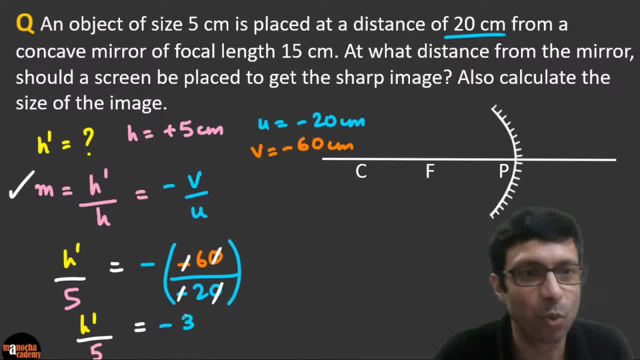 excellent. not three guys minus three, right. and so what is the final answer? you just take five on the other side and therefore we are getting h. dash equals minus 15 centimeters is our answer here. are you guys getting that minus 15, right? so what does this? 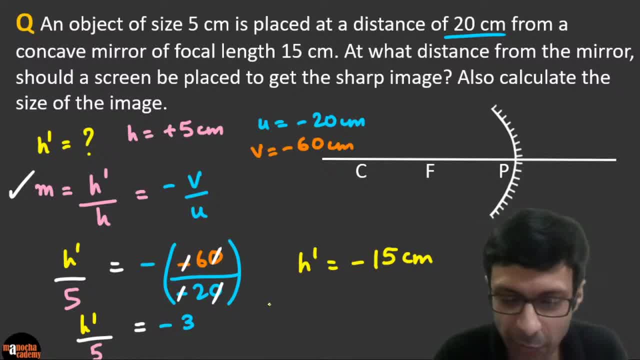 tell you about the image: right, The image height is minus 15, right. So image height is basically we can say 15.. So image height is 15 centimeters and it is the minus sign tells you it is inverted. and it is inverted right Because it is along the negative x. 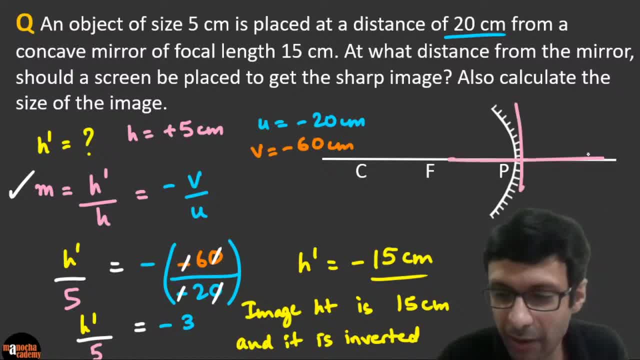 axis. Please remember, the axis were like this: right, These are our axes. right So x axis, x dash, and you have y and y dash, right. So the image is formed. it is inverted and it is formed along the negative x axis, That means negative y axis, sorry. So it is inverted. 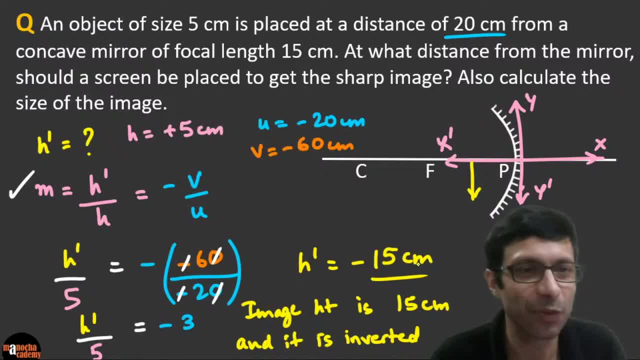 Very good. I see lot of you have written minus 15 centimeters. Srihari has the correct answer. Don't forget centimeters, guys. Don't forget the units. Awesome, Great to see you guys are enjoying. Please hit the like button right now. If you haven't hit it already, we will. 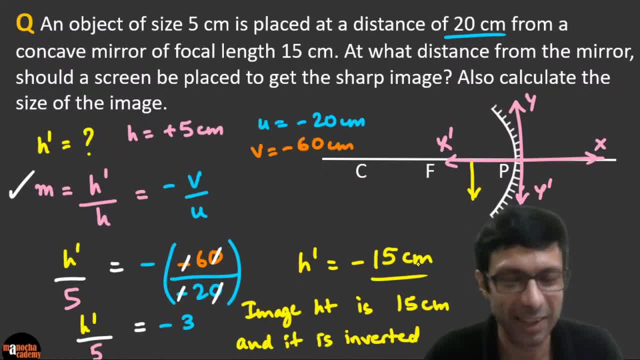 be at 500 likes. I think Awesome guys, Is it clear? So this is how you do it: Draw the diagram, write down the formula and substitute. It will be very simple for you, Awesome, Great. And here is the final. 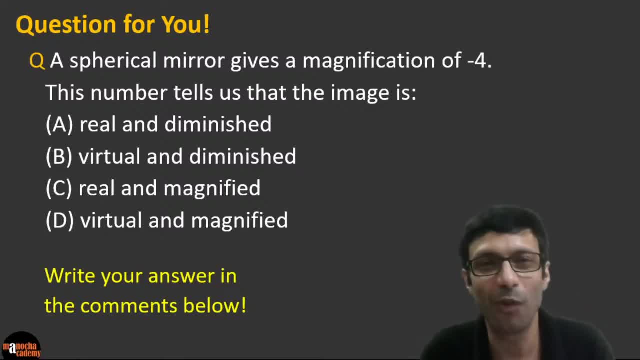 question for you, which is going to be the homework question. Thanks guys, We are over 500 likes. Thanks a lot for your love and support. And here is the last question. A spherical mirror gives a magnification of minus 4.. Now, what does this number tell us? 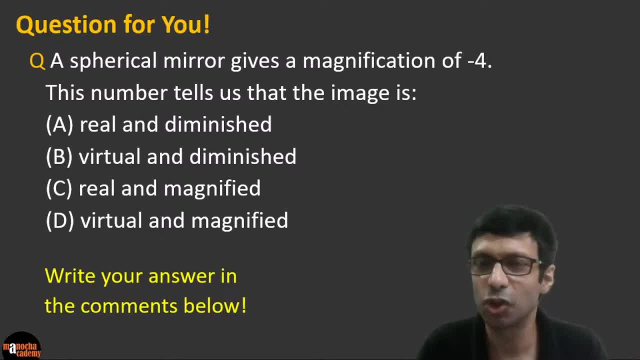 Is the image real and diminished? Is it virtual and diminished, Or is it real and magnified? Or is it virtual and magnified? What do you guys think? And I am not going to tell you this answer here, because I want all of you to think and try and do write your answer in the comments below and I will definitely. 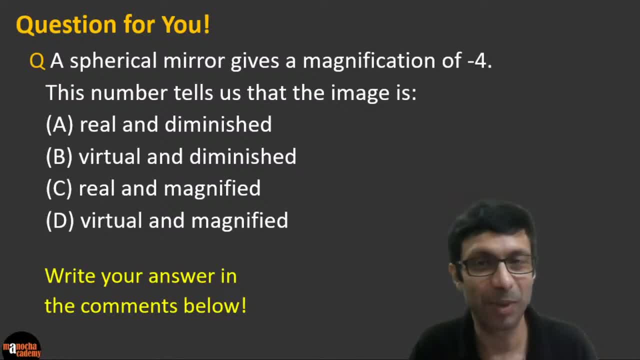 reply to it as soon as possible. So, guys, please try this question. Interesting question We have been given the magnification is minus 4.. What does this tell us about the number, The magnification number? it is a very important question. Often it is asked. 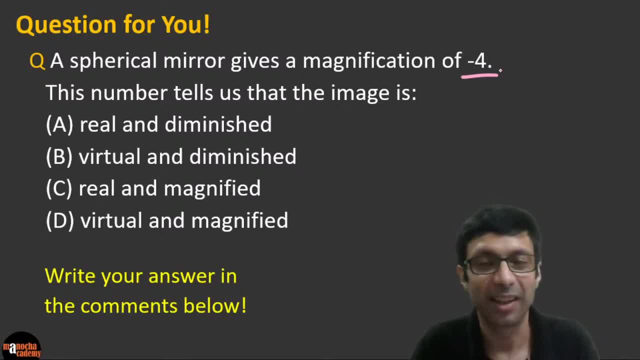 And I told you in this class I am going to discuss some really important questions that will help you clear the concepts and for you to do better in your tests. So please try this question and please write your answer in the comments below, because I won't give. 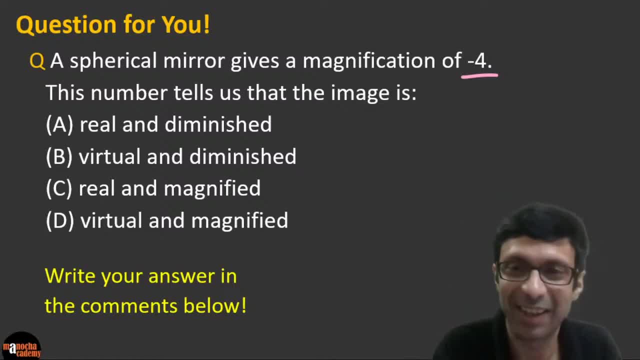 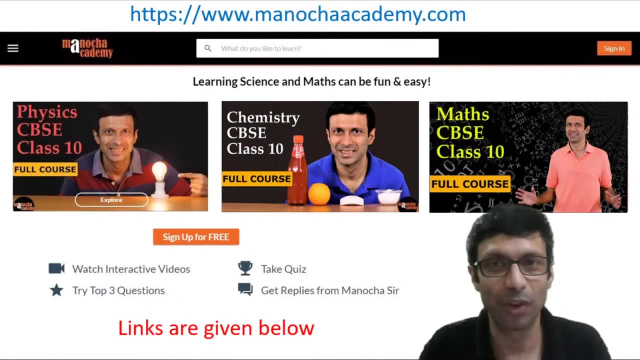 you the answer right now. I want everybody to try And guys, as I said, do check out our website manochacademycom. You know I take more live classes over there. We have interactive videos, quizzes and questions and you get direct replies from me, So definitely. 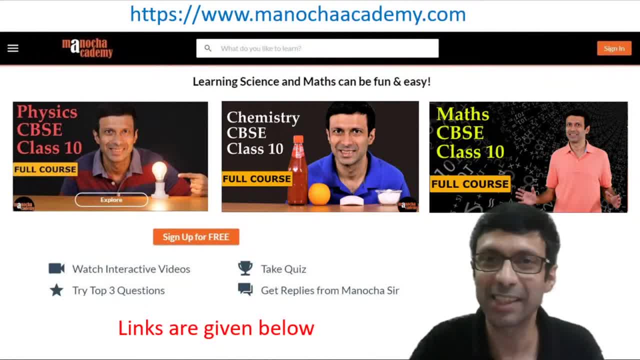 guys do check out our website. We have these full courses for physics, chemistry and maths on our website for CBSE class 9 and 10 and for ICSE, class 9.. And guys do share it out with your friends, Okay. So thanks a lot. Hope you enjoyed this class and please hit the like button. 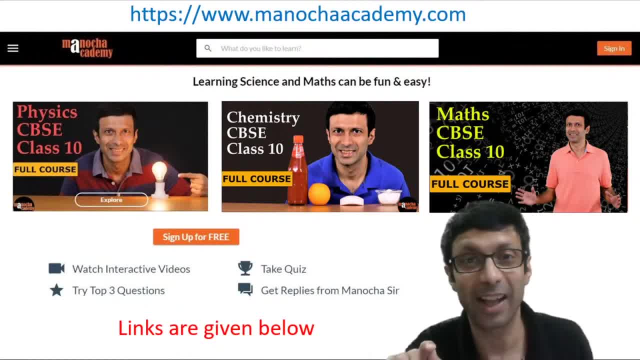 and also don't forget to hit the subscribe button and the notification bell so that you don't miss any of our videos or live classes, And I'll keep taking these, you know, classes on our Manochacademy English channel, this Manochacademy channel, and I've also started Hindi live. 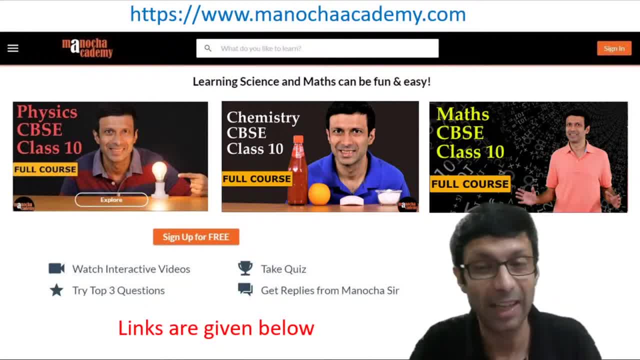 classes. if you guys are interested on Manochacademy Hindi, So you guys can search for Manochacademy Hindi and hit the subscribe and notification bell and do share that out with your friends. So I'll be taking you know some. probably there'll be a Hindi class tomorrow or day. 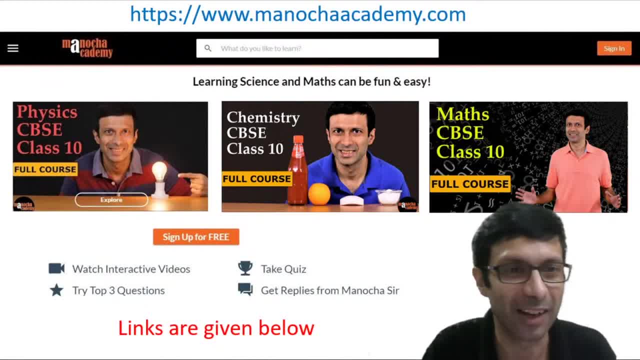 after: Okay. So, guys, if you're interested in that, do sign up for that. Awesome guys, Awesome. Hope you enjoyed the class and do take care of your health. Thanks a lot. Yes, Thank you. Thank you. It's like 525 likes. Awesome guys. Great to see the response. Hope you found this. 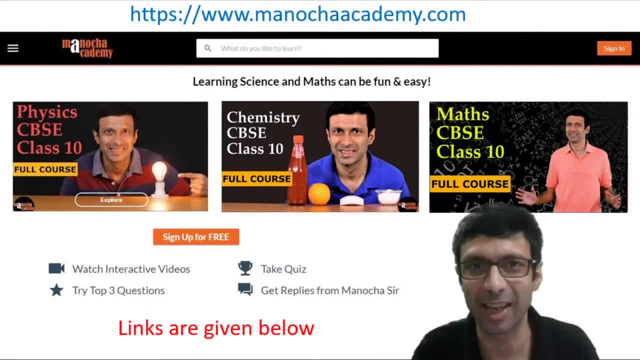 class useful and helped you revise many, many important concepts, and I'm sure you guys will do well. Just keep studying, keep the momentum going and all of you, please work hard. I know this is a difficult time, but it's an opportunity to learn and please take care of your health. 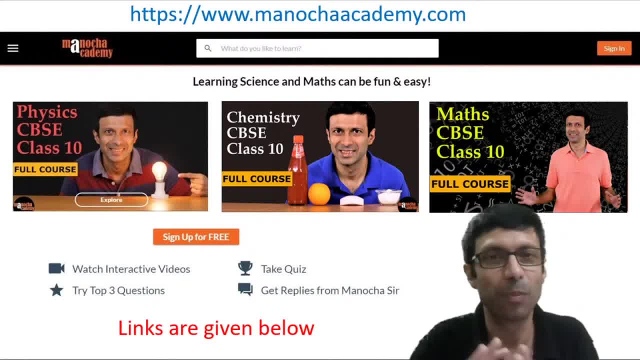 keep a balanced life. Don't be just studying or don't be, you know, just relaxing. Keep a good balance. You know that's always my suggestion: Keep a good balance, and I'm sure all of you guys will do well. 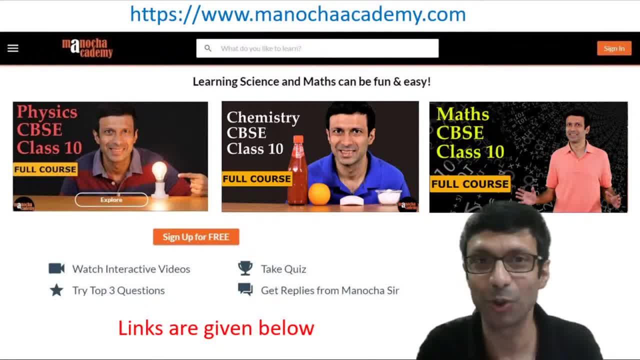 Thanks a lot for joining in the live class. So this is Sandeep Manocha signing off, and see you in the next live class. whether we have it on our English channel, Manocha Academy, or the Hindi channel, I want you guys to be there and do share it out with your friends. 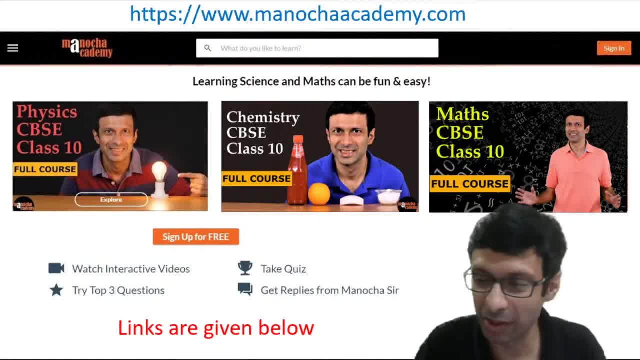 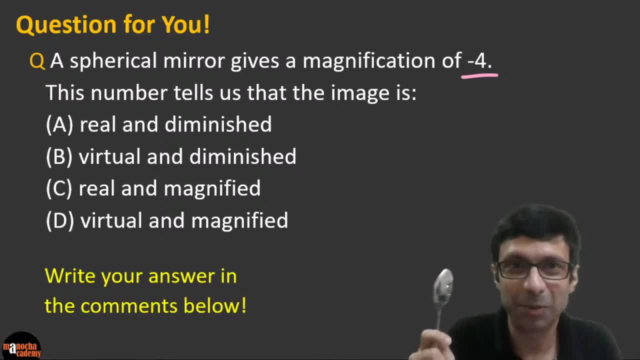 Thanks a lot for joining. Oh, and don't forget- you know I mentioned, so don't forget to do this homework question. and, guys, when you are having lunch or dinner or your breakfast, please pick up that spoon, right. it is the best example of the concave mirror that you have at. 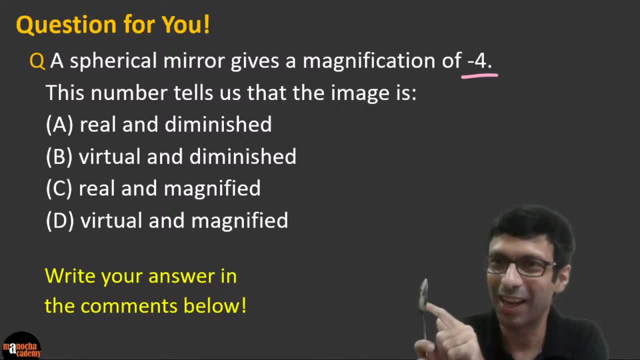 your home and you know the best part: it has both a concave side and a convex side. right, you have a concave mirror- the front portion- and a convex. okay, so carefully, look at the image that's formed in the mirror and i'm sure that will help you remember many things, because remember convex. 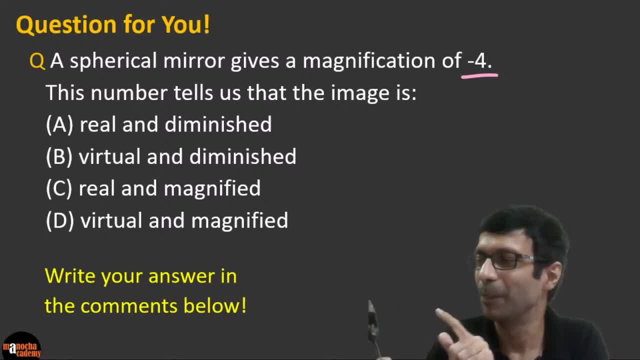 mirror always gives an upright image, the back portion and the front. one can give an upright or a inverted, because it can form both real and virtual images. awesome guys, awesome, great to see the response and see you in the next live class and do share it with your friends.